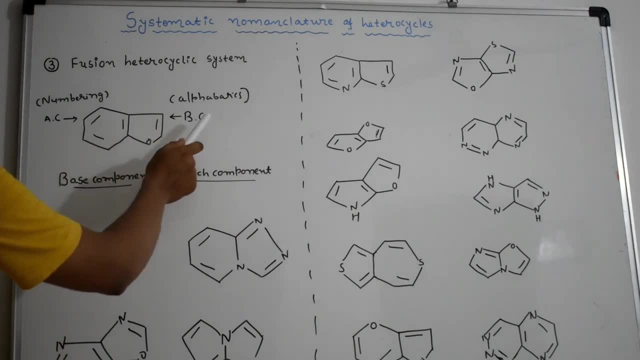 it will come first, Your base component will become second and your attached component will be your graphics. So here, the first is a benzene ring, so I will write benzene. So we have to E? n, put the O instead of your E, so benzo. then we have to put the square bracket. 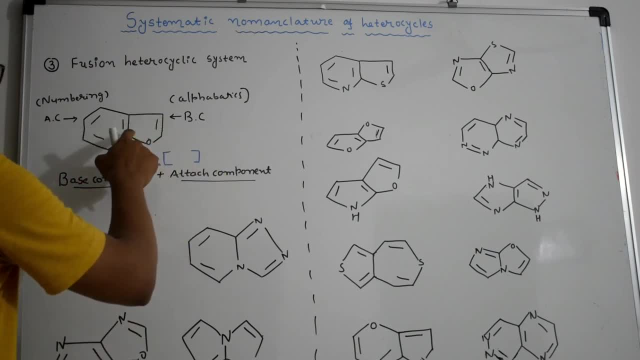 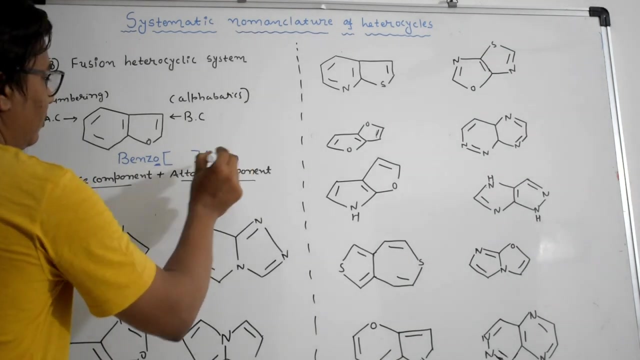 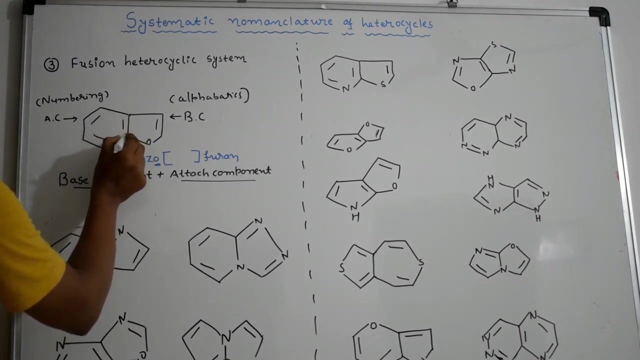 then your base component is a furan, and if it is not, a tribal name is available, then we will do the systematic noun that we had studied, the hands with men. so here we have to write the furan. now we have to show the attachment, so occupant start with the. you have to give the minimum, no possible number to. 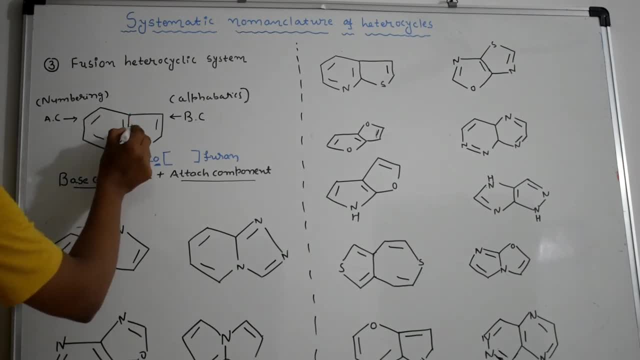 this attest one. so here I review A, B, C, D, any so parties from the position B. so here there is no requirement to give the numbers to the bend in between, for the behavior can attack from the any position, so it will be benzobifuran. so 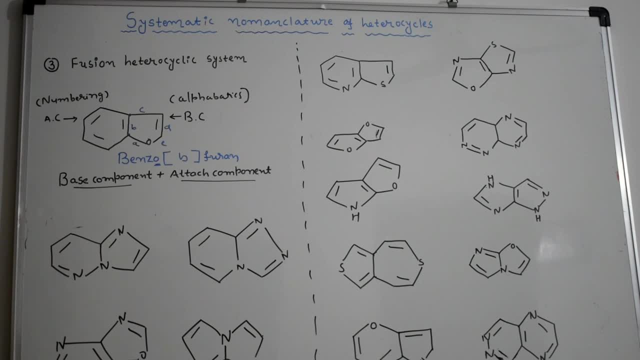 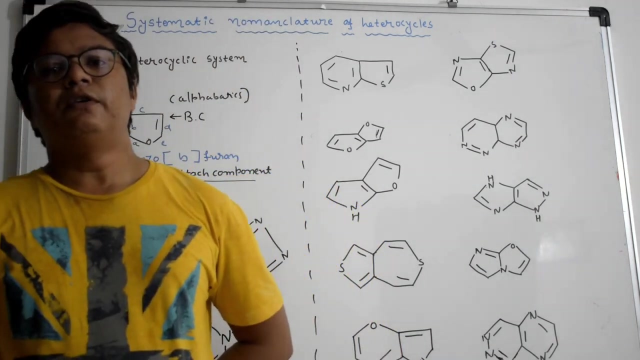 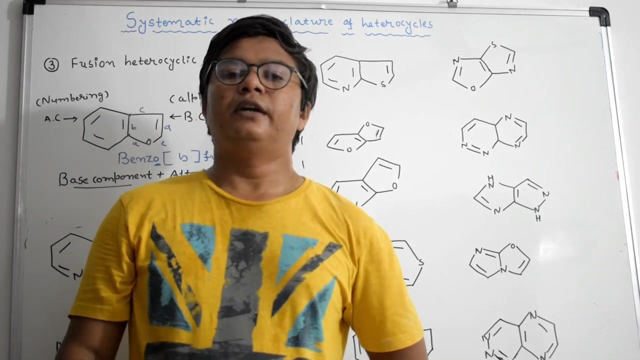 now let's go on. really, another example, therefore. we are taking this example, right men will take this example. so first we have to identify which one will be the base component. so for the base component, what we will do: first we have to see the body. if any ring contain hydro atom right other than the nitrogen, then we 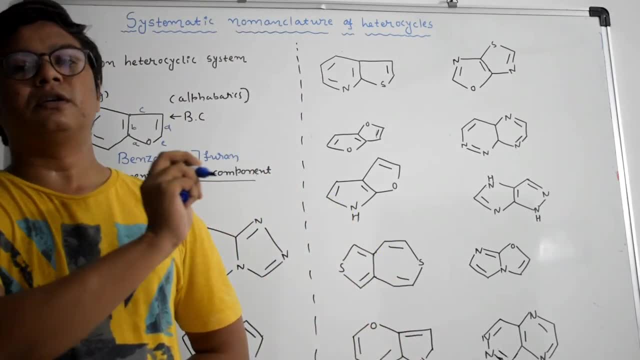 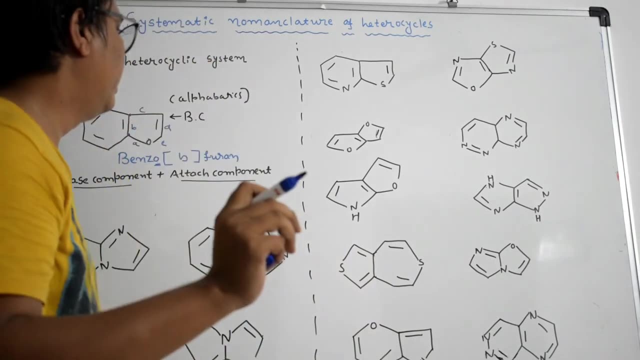 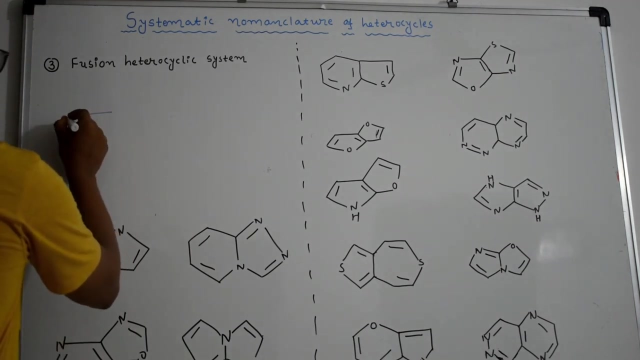 will be called right, it will be as a base component. if nitrogen is there, then the ring which contain a nitrogen atom will always called as a base component. so I will take you every taking one example, like if you have, like this is one ring attached with another five member ring, now this: both the ring contain the 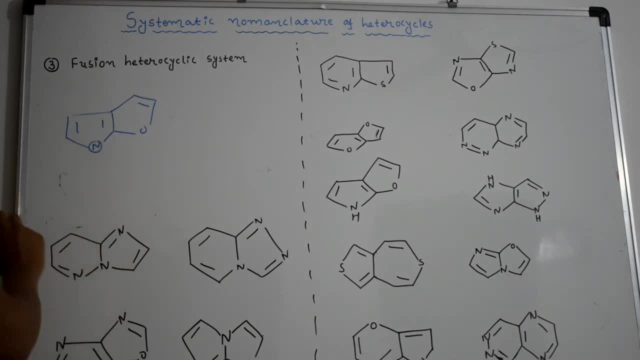 hydro atom, but the ring which contain the nitrogen will be called as the base component. so first we have to check whether there is a nitrogen or not. ring which contain the nitrogen will always called a base component. if the is no nitrogen and other than nitrogen hydro atoms are there, then we have to check that. if 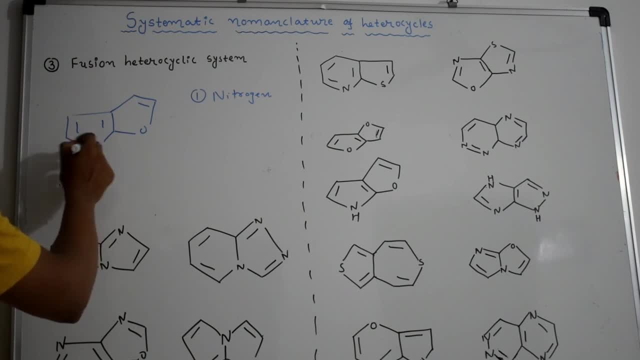 there is no nitrogen and if there is a sulfur, then what we will do? we will go by the order of electronegative which we had discussed in the previous video, such as oxygen will come first, then sulfur, then nitrogen. right, like this thing. so in this order, oxygen come first, so this will. 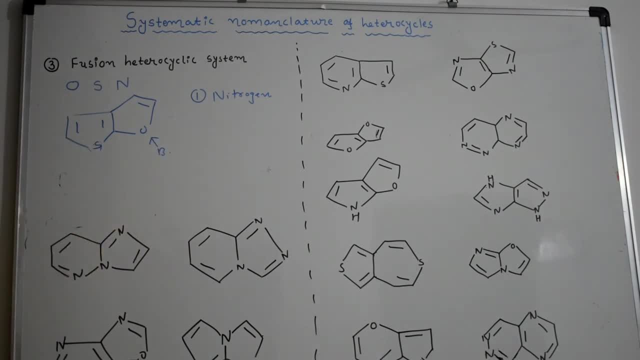 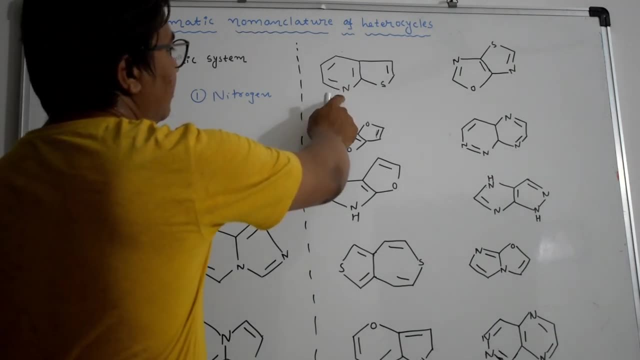 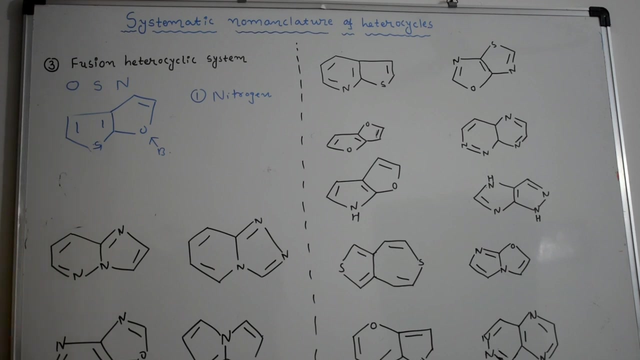 become your base component and this will become your attached component. so, for this ring, the nitrogen containing ring is there, so it is became your base component and this will become your attached component, right? so, as we will go with the example, then what we will do then we will. 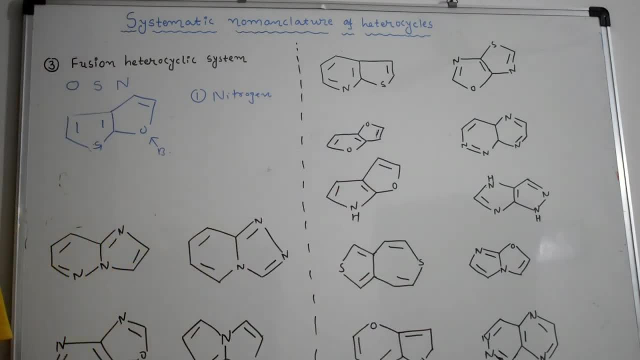 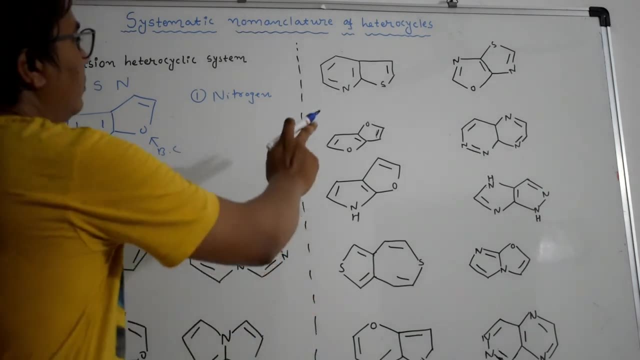 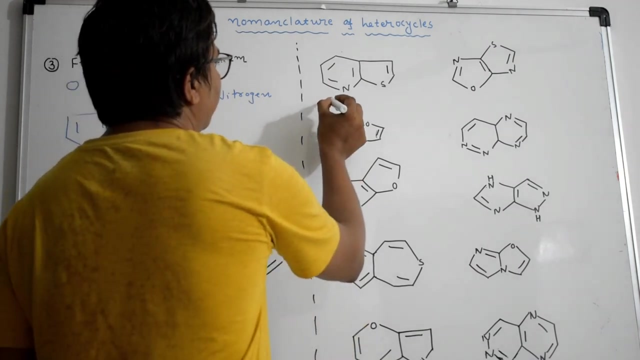 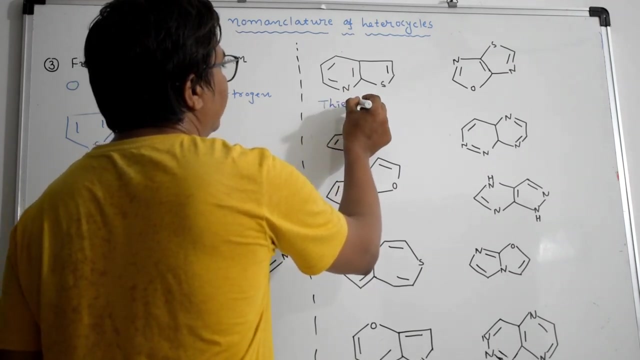 see the rule for the each example and we will understand it. so this is your base component and this is your attached component. so now let us solve this example. this one is your base component, this one is your attached component. so, for attached component, it is a thiophene, so it will be written as thi-eno. it will be written as thi-eno. this is square. 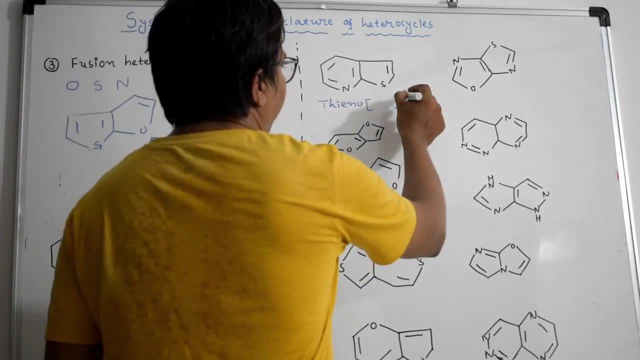 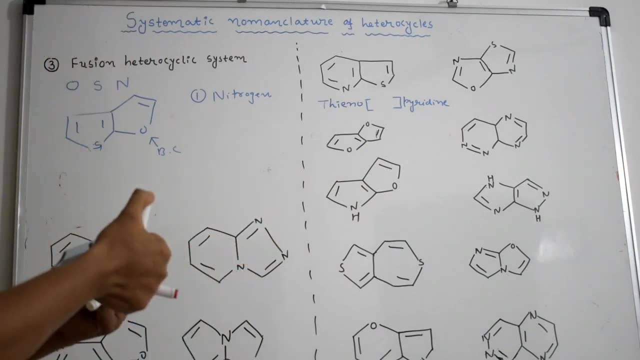 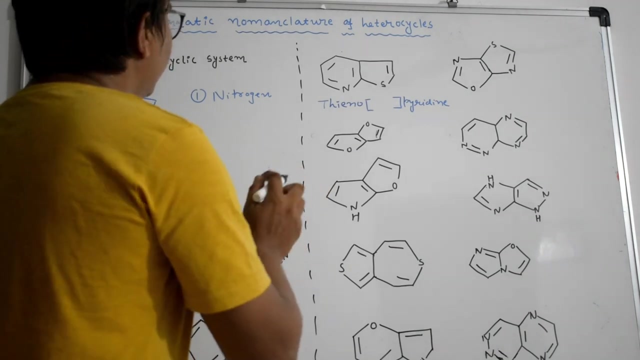 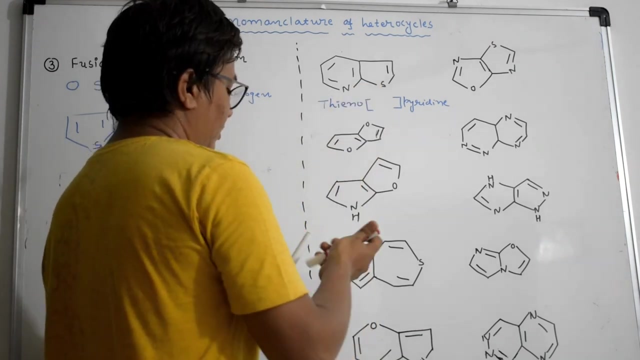 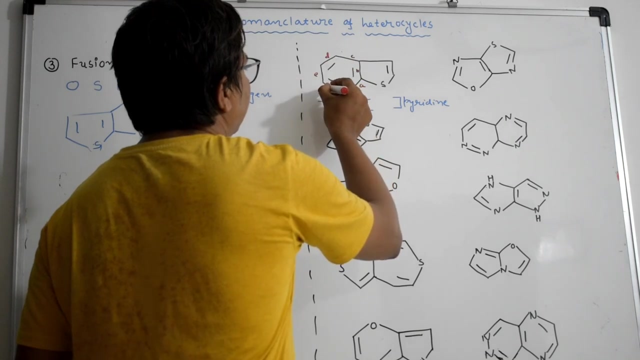 bracket and the base component is pyridine. so here i will write pyridine. now there is a time to show the fusion right. so how we will show the fusion for the base component, what we will do for the fusion, is like a right. it starts with the a, here it is b, c, d, e and f, for this is a sulfur atom. now 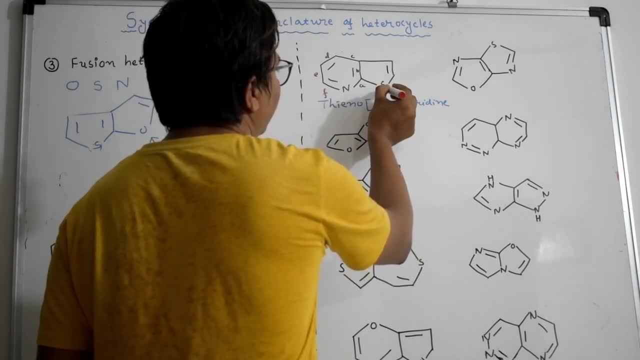 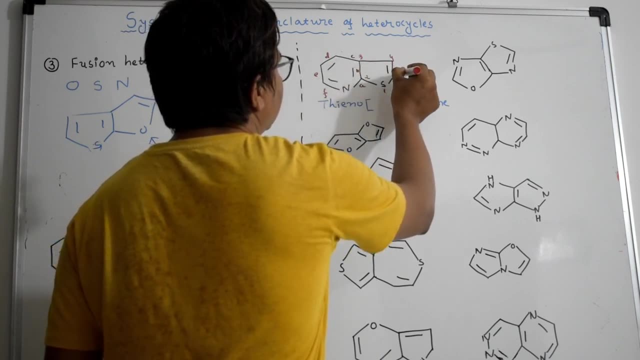 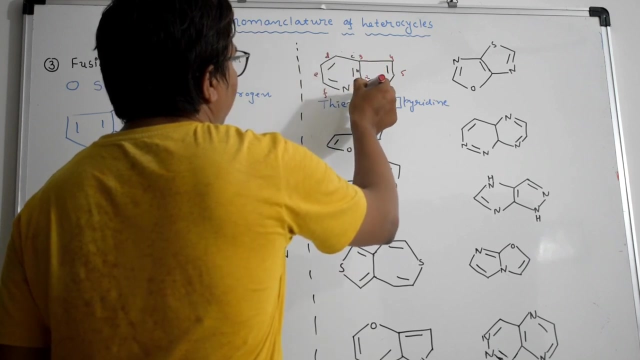 i have to give the number to the attached atom. so how? how i will go? i will give the first number to this, second to this, third to this, four to this and fifth to this. so you can see your alphabet is right. it is going in this direction and the same way, your numbering is also going in the same. 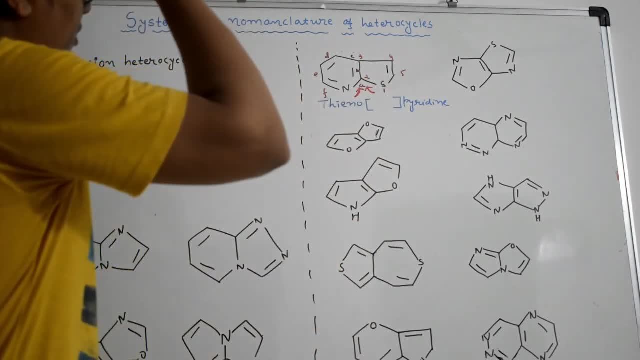 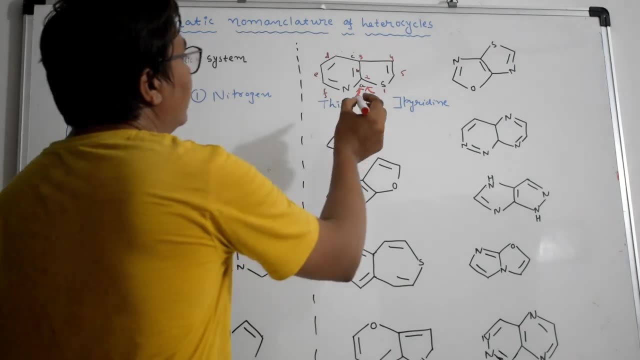 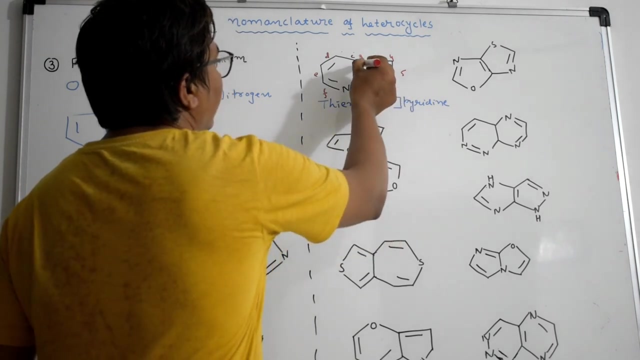 direction, it should be the conjuring, it should be converging and it means that it goes to the in same side. so here, from which number it is attached, you get two and three, so numbering will come first: two, three, and the one is b, so it will become two, three, b, so it's iotc in. 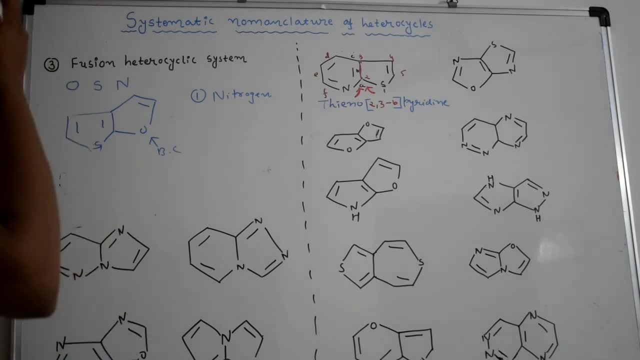 will be Tai Inoh, two, three b pyridine. now let us have the another example, this one right. for this example you can see the both the ring are same. so for the same ring you can consider anything as a base component and any ring as the attached component. so this is no matter of choice. 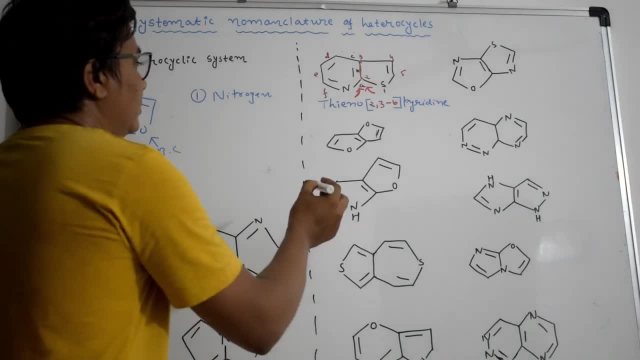 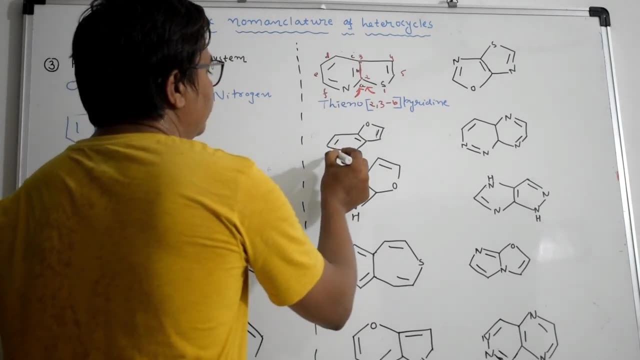 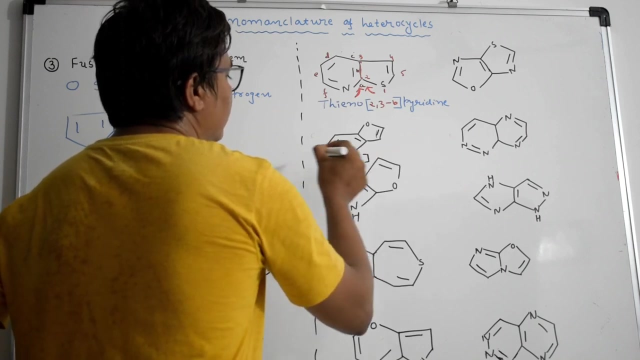 that, whether to which one is a base component, at which one is attached component, say, for example, here I am taking: this is the base component, so it anywhere will go. there will be become is a furan, so it will call as a furu right square bracket and this is. 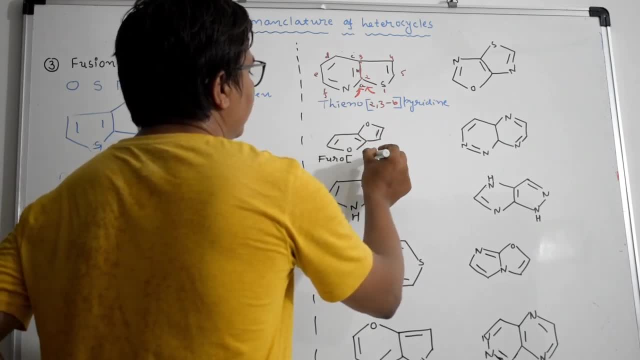 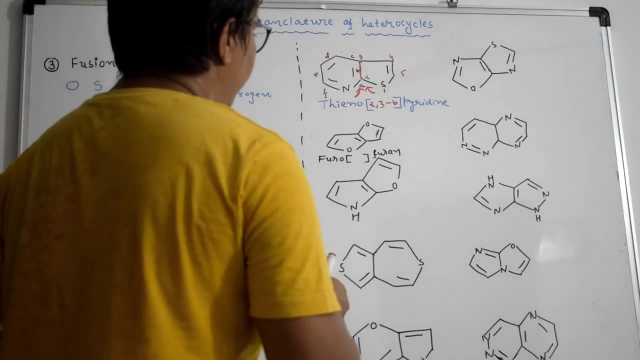 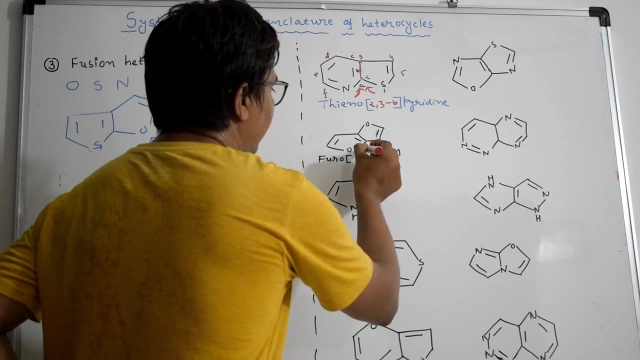 your base component, attached component- will be furu. so it is a furan now. so the one ring which I have assumed as the base component, I will give the alpha particle order. so here I am taking it as the base component. so A, B, C, D, right now. 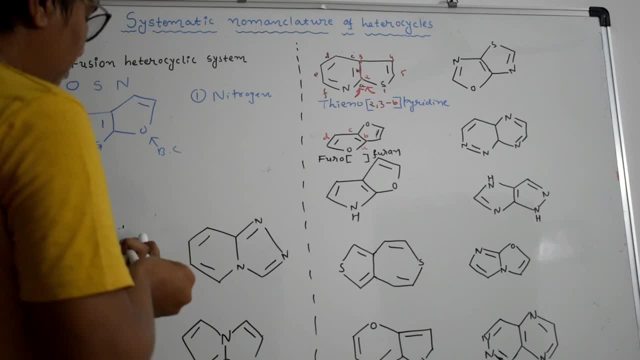 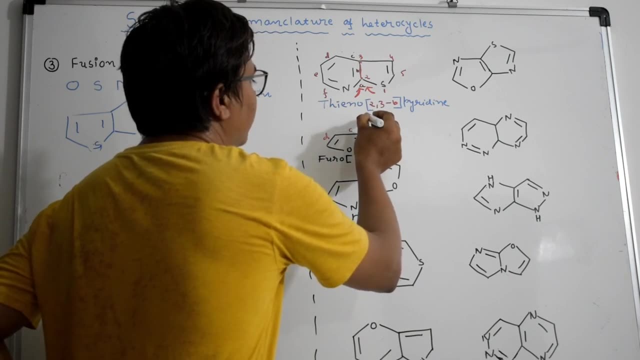 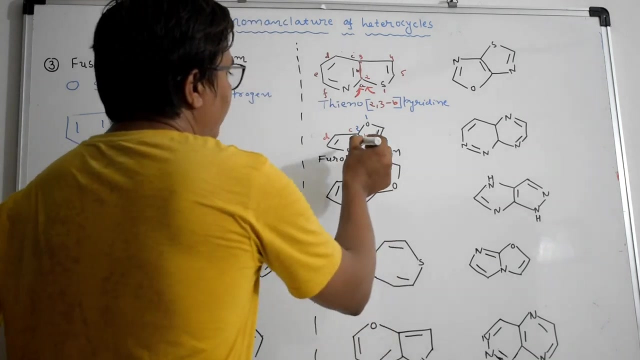 for the attached component. I have to give the numbers, so numbering starts from that. so first I have to give the number to the heteroatom right. always numbering starts from the heteroatom. so 1, 2, 3, 4, like this: now you can see your alphabet. 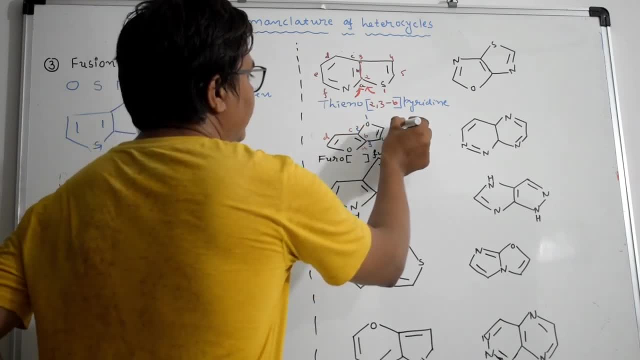 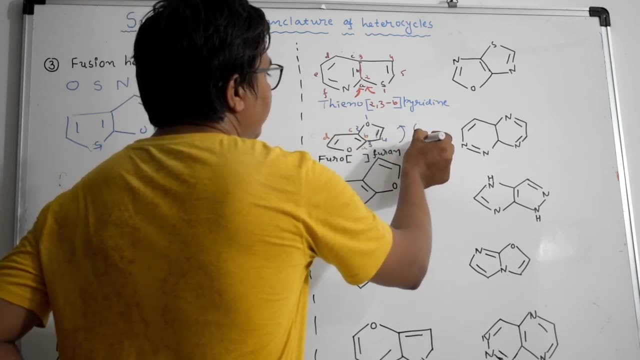 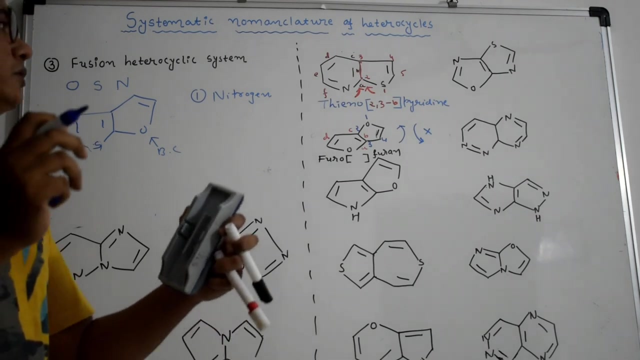 is going like this: a, B, D. which direction is this? and your numbering is coming like 1, 2, 3. your number is coming like this: so this will not be work here. so what we have to do, we have to take it should be in a, your converging direction. it will be into the same direction, right? so what i 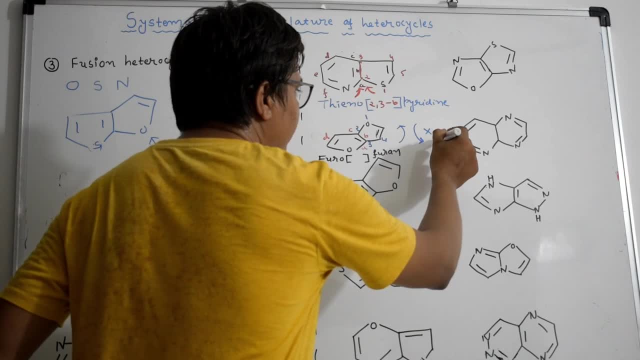 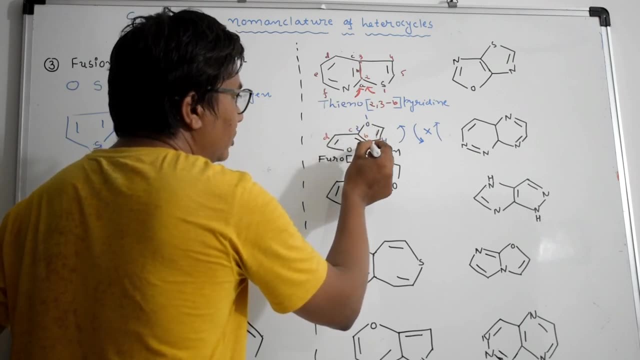 have to do this number. instead of this, i have to take the direction like this. so here, if i will put A and this B, so 2, 3 will not be position, but instead of 2, 3, i have to take a, 3, 2 right, because this will come into the opposite direction. i have to take the both. 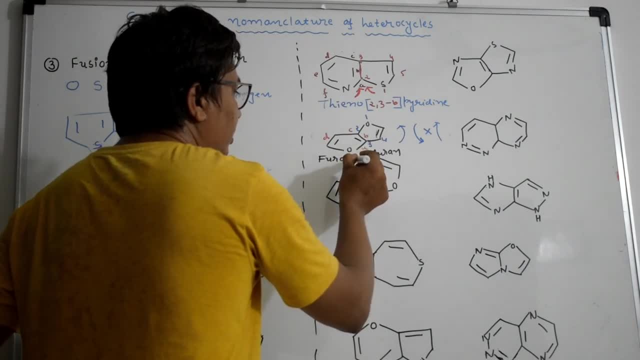 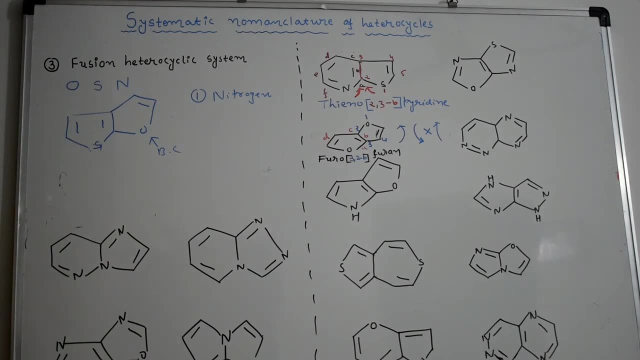 the direction same. so it will written as a 3, 2 B furan. right, it will be written as a 3, 2 furan. so now let us see the third example. so in the third example you can see the both the rings are five numbered ring. 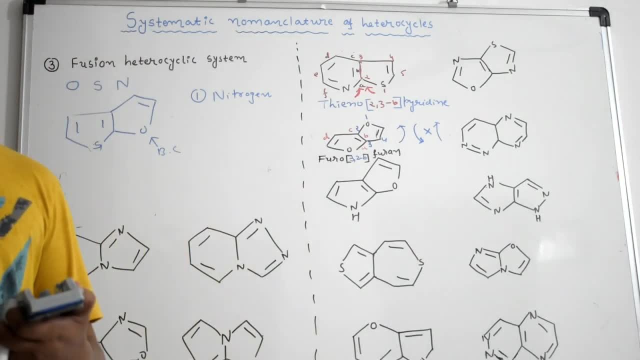 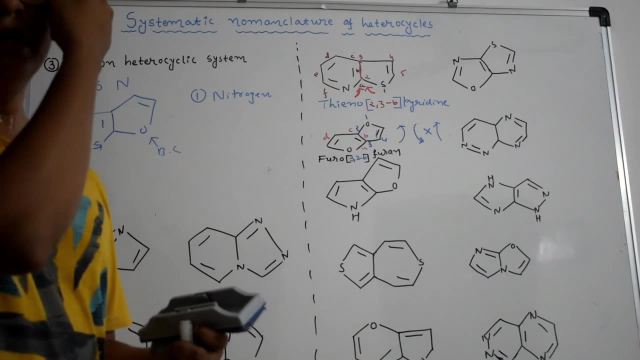 1, 2, 3, 5. One is containing oxygen as a heteroatom and another is containing nitrogen as a heteroatom. So, as I have told you, when you compare the ring, when nitrogen ring is there, it will always become your base component. 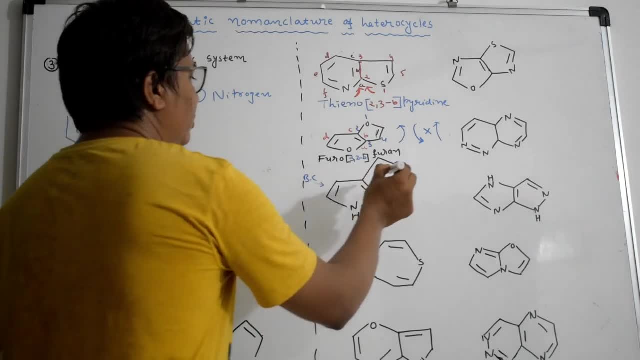 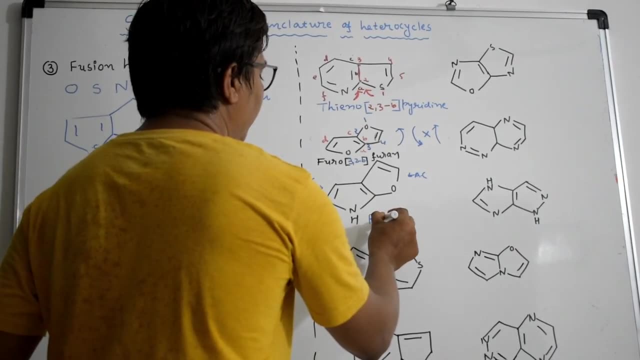 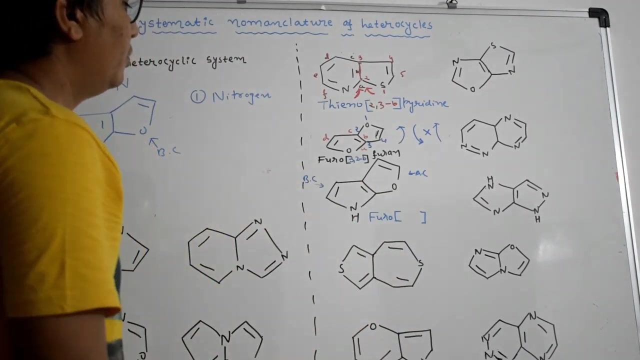 So here it is your base component and here it is your attached component. So attached component is your furan, So I will write furon, Hope you will understand Furon Square bracket. And this is what For this molecule, the tribal name is present. 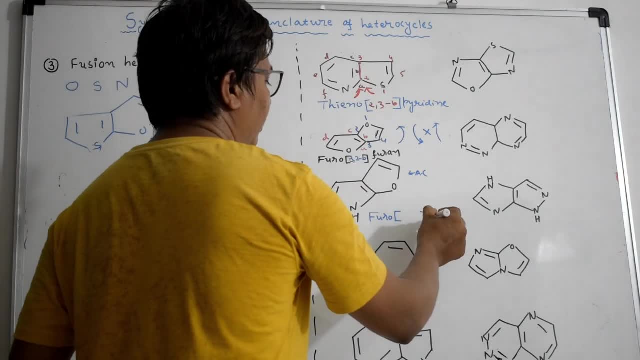 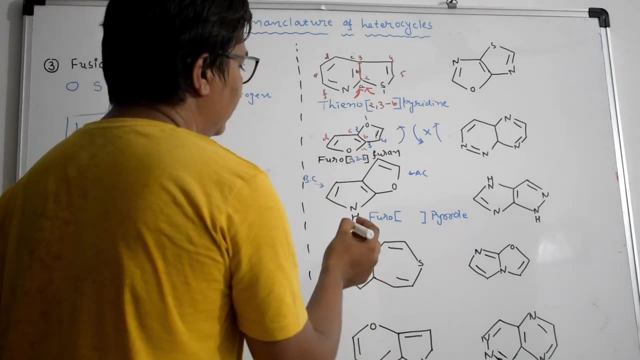 So you have to write pyro. Its tribal name is pyro, So I will write pyro. Now for the base component. what we have to do? Give the alphabets, So A, B, C, D and E. 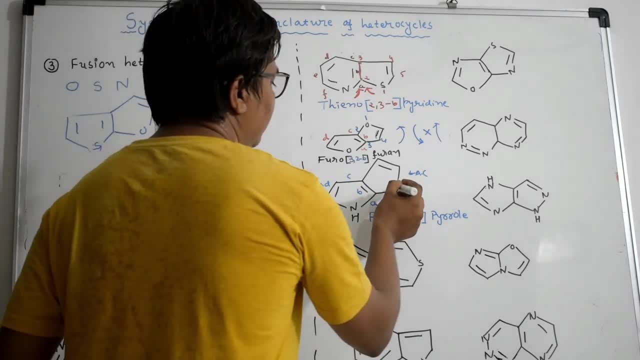 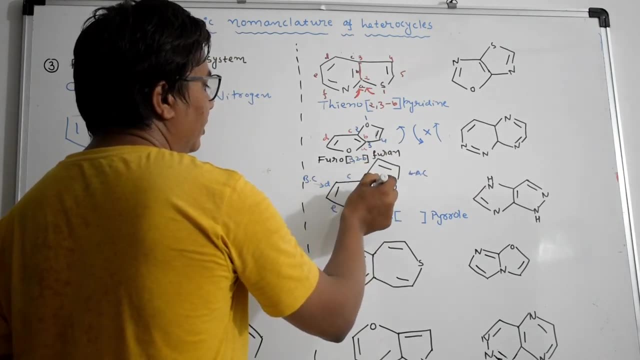 And for the attached component. we have to do numbering. So numbering always stands for the heteroatom And we have to give the. We can't go on this side, Because if I will go on this side, it will get the greater number. 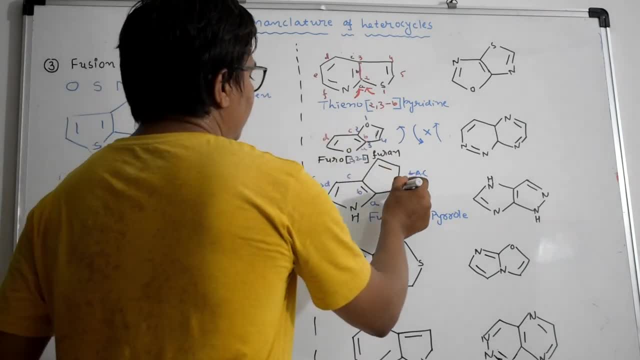 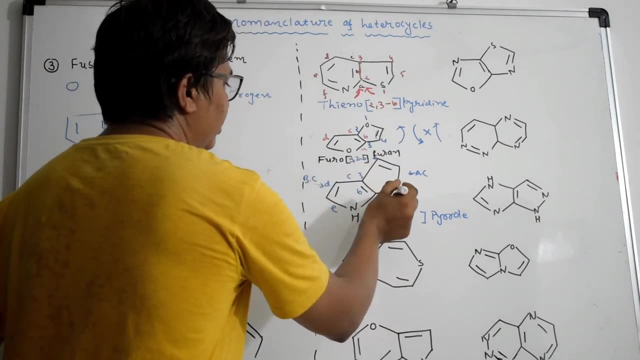 We have to go this side, so it will get the smallest number, So 1,, 2,, 3, 4.. Now check the direction: A, B, C going this direction. 1,, 2,, 3 going this direction. 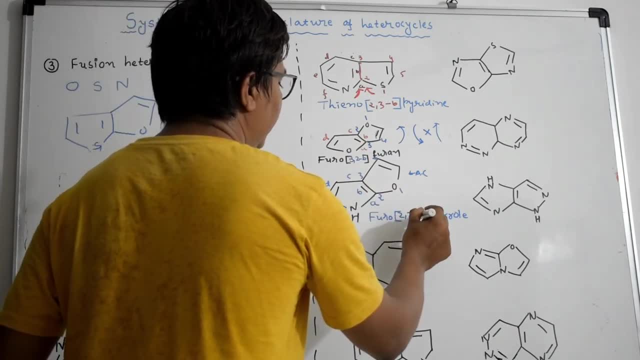 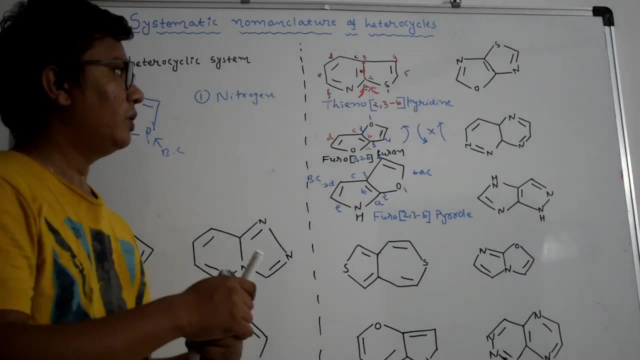 So you have no need to change. So I will write 2, 3, B. Write furon 2, 3, B, pyro, Now, let us. So. now let us discuss this example. 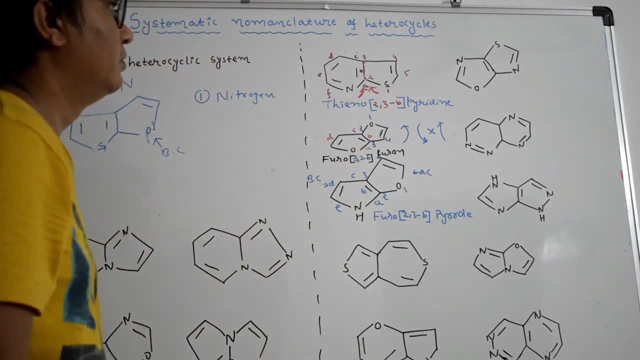 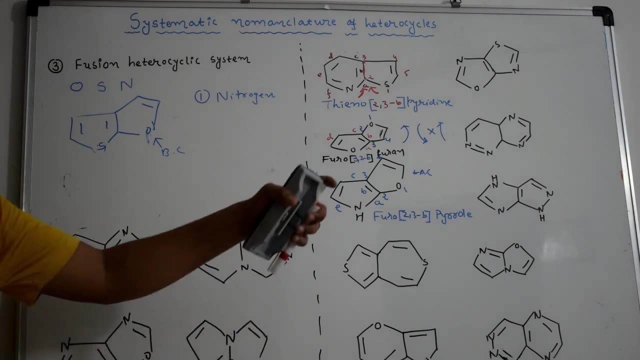 Here again, the two ring And the far number ring Right. So now both the ring containing the nitrogen atom Right. So what we had seen previously, that if your ring is contained in nitrogen atom, it will be called as the base component. 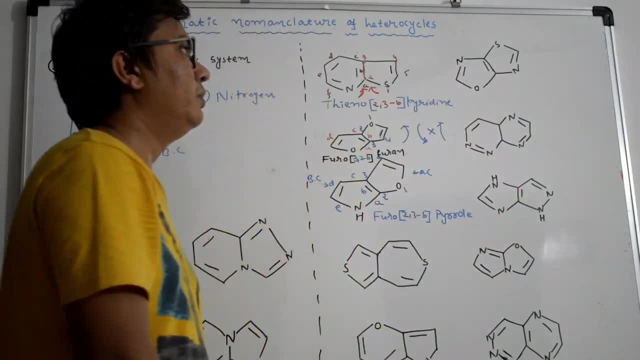 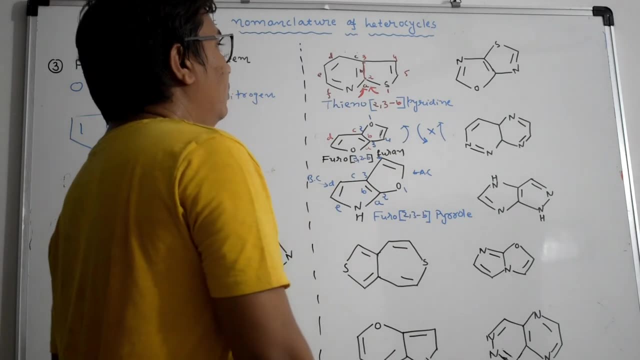 But here both the ring containing the nitrogen atom. So in that case, what we will see? We will see the other atom. The other atom is sulfur and oxygen. Now, in that case, again, we will see the priority: Oxygen comes first in the sulfur. 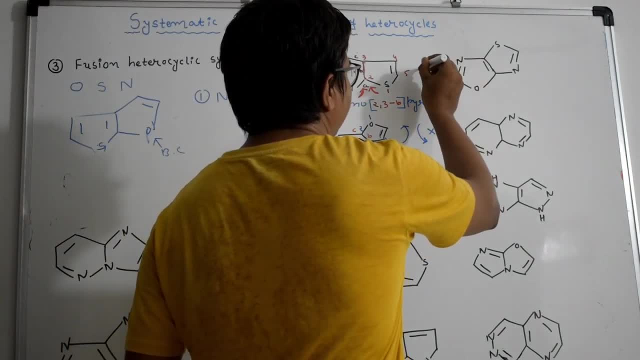 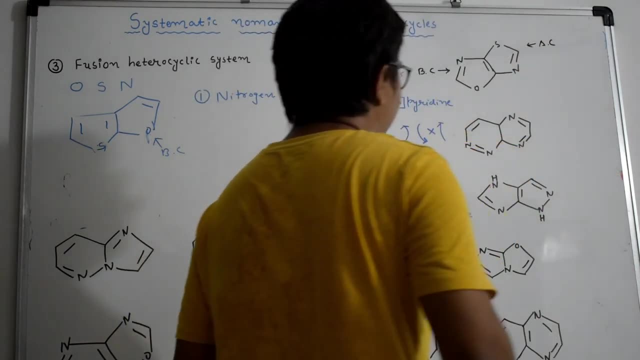 So your this ring will become a Base component, Your this ring will become a base component And your this ring will become an attached component. Now what we will do for the base component and attached component. we will write the name for this. 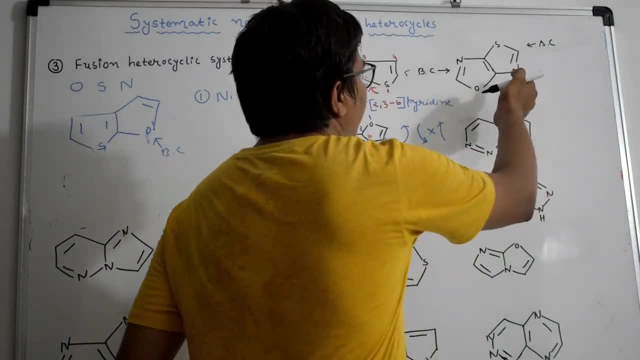 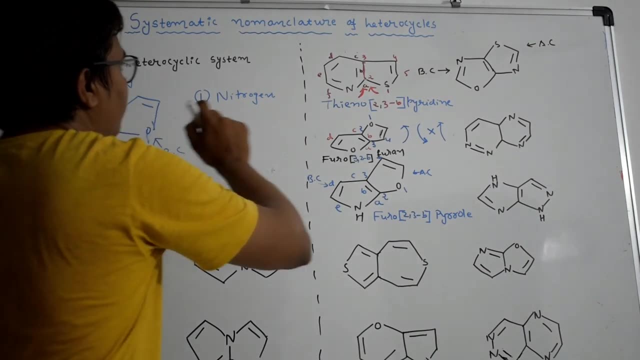 Right, So for this component, what will be the name? You can see that they are on a one-third position of each other. So here, in this sequence, sulfur comes first, So it will get the first number. So I can write it like this way: 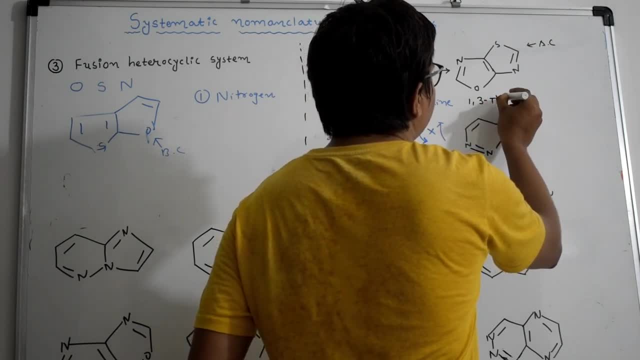 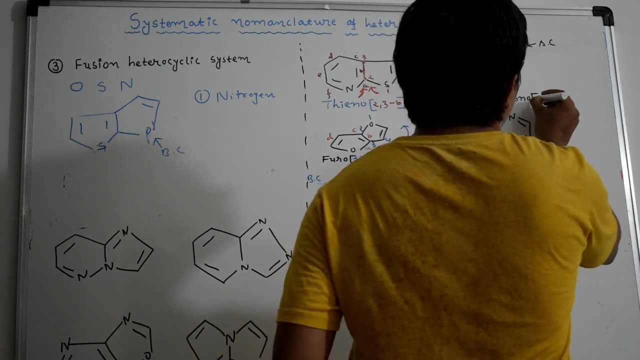 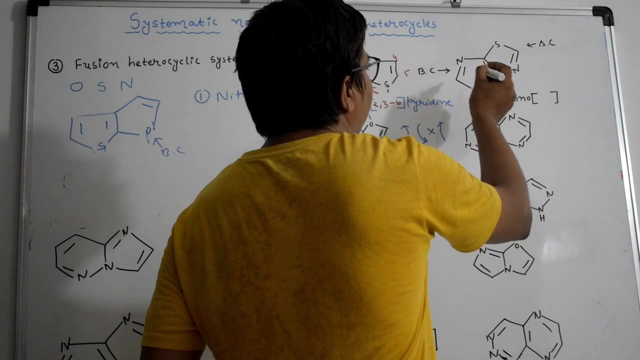 1, 3.. Right Thi-azeno, Right, Thi-azeno. Again, it will be on the square bracket And your this ring is again on a one-third number. Your oxygen and nitrogen Right, And the oxygen comes first. 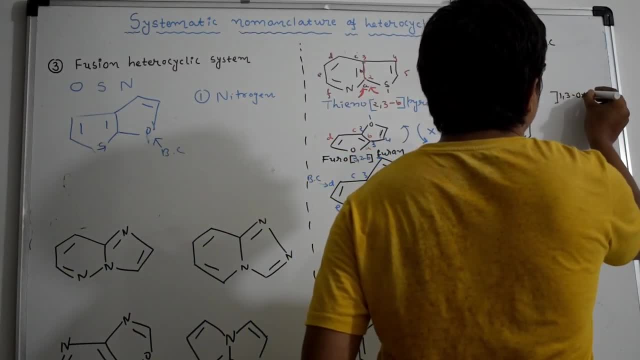 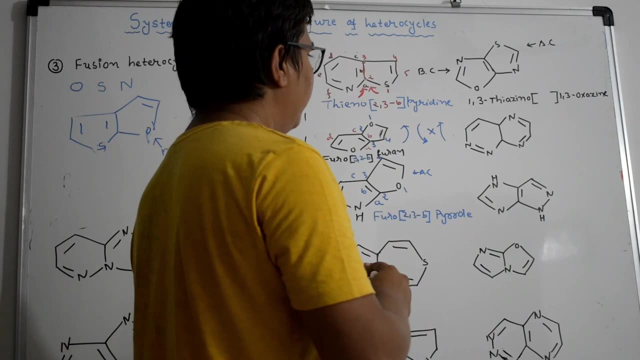 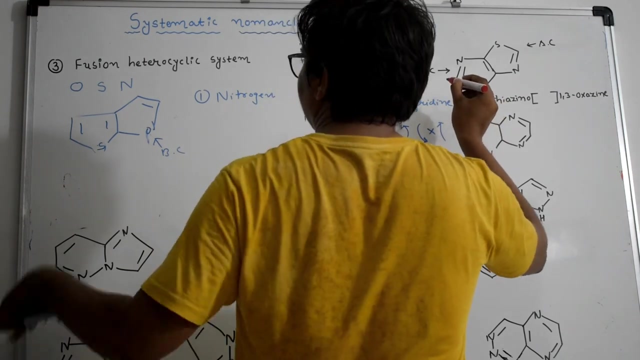 So I will say oxazine, Right, Ox-azine, Now. Now. Now what we will do. we will give the alphabets to the, your base component. So from where it will be? start from oxygen atom, because it comes first. 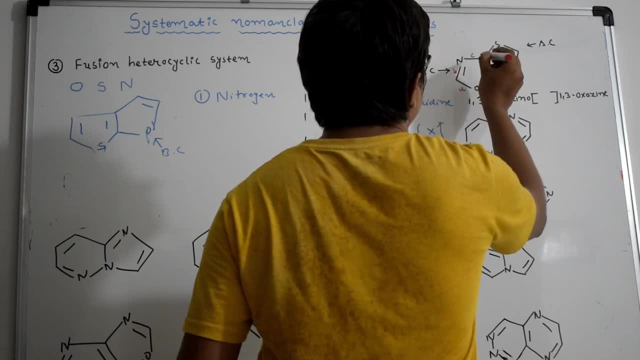 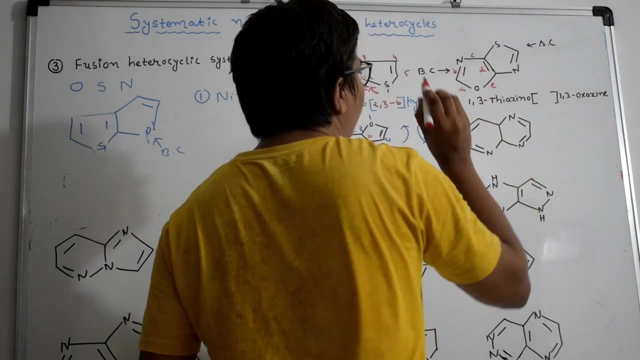 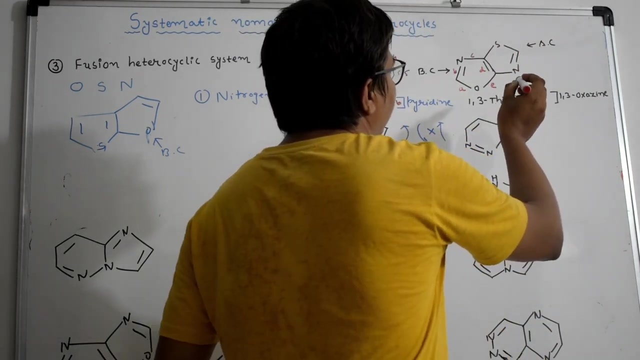 So here A, B, C, D and E. I can't go in this direction because your bond nearer to the heteroatom gets the lower alphabetical order. Now for the your this attached component, we have to give the numbering. 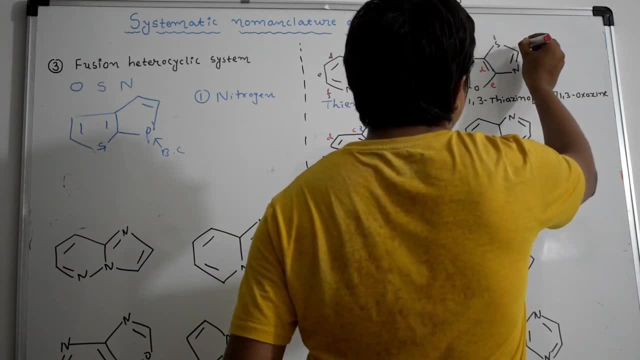 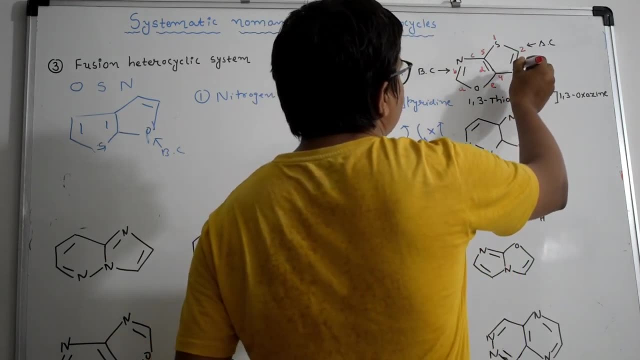 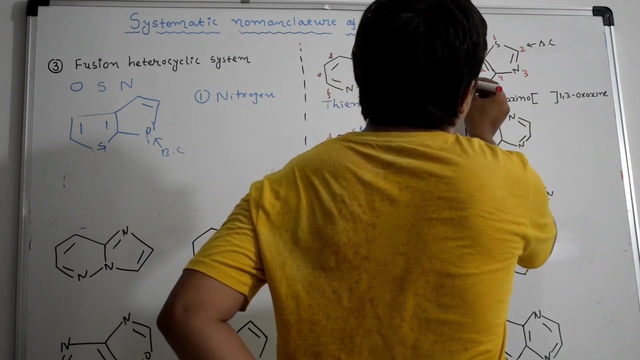 So sulfur comes first. So I have to go like this: 1, 2,, 3,, 4 and 5.. Right, I can't go in this direction because this nitrogen should be get the lowest number. So here you can see. your alphabet is good playing this: A, B, C, D, E. 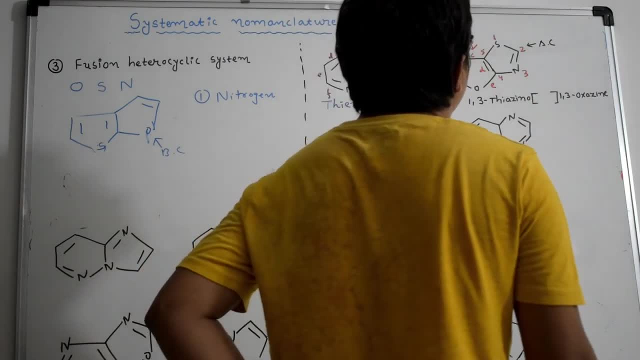 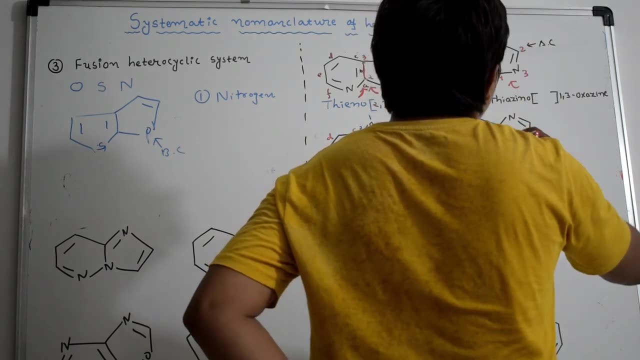 It's going on to this direction and your numbering going into the this direction: Right: 1,, 2,, 3,, 4, 5.. So it will not work Again, because it should be a into the same direction. 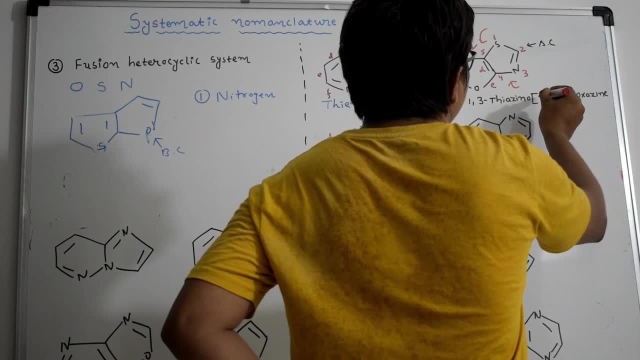 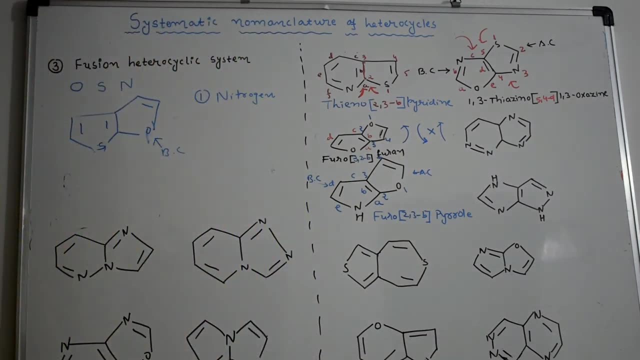 So I have to take from this direction. So it will become 5, 4, D. it will become 5, 4, D, Right? So let us take the another example. Another example: we are taking this molecule. 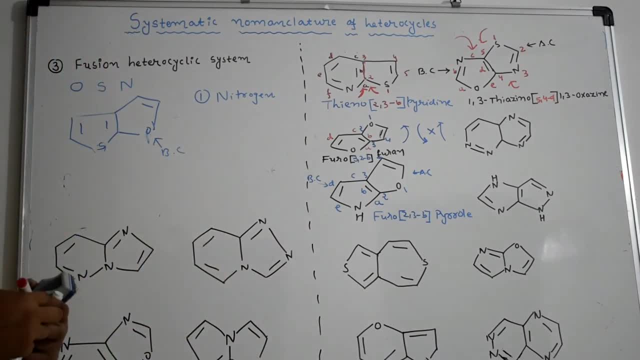 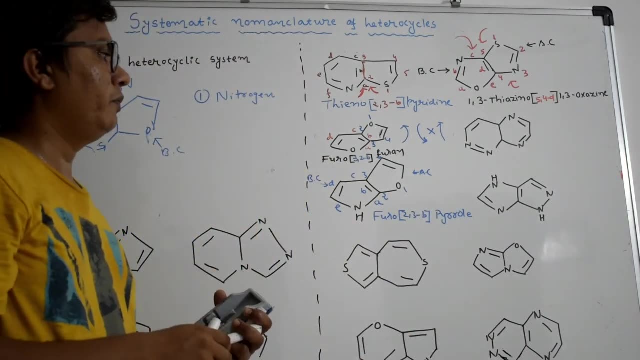 Right For this molecule. you can see that both the rings are have equal size. both are the five member ring. Both contain the equal numbers of nitrogen Right. So this is the nitrogen atom. So what we will, how we will decide the base component in that case. 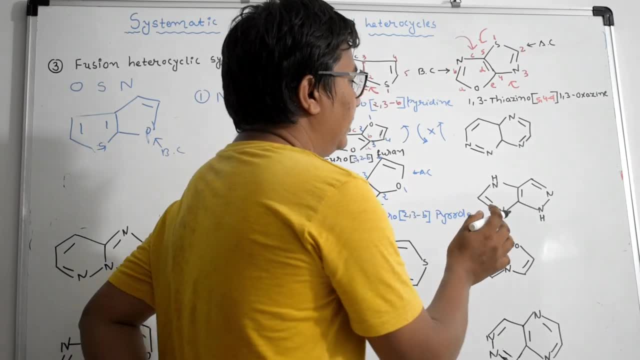 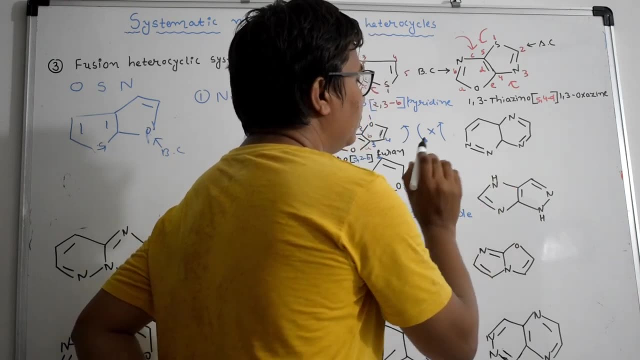 For in that case base component will be: decide that lowest locate number. So here you can say the two nitrogen atoms are 1, 2 and 3.. 1,, 2, 3 from the each other, and here you can say they are on to the 1, 2 number. 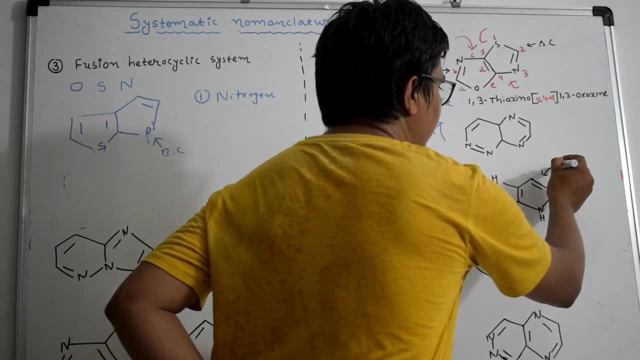 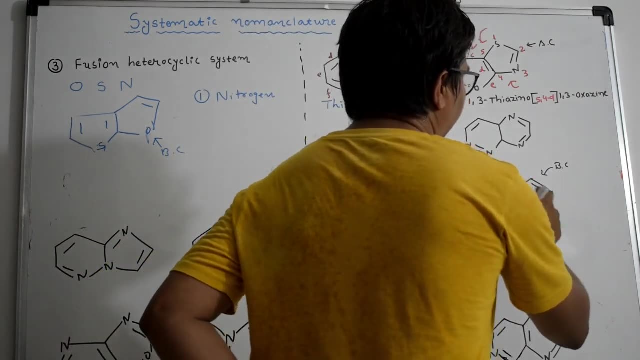 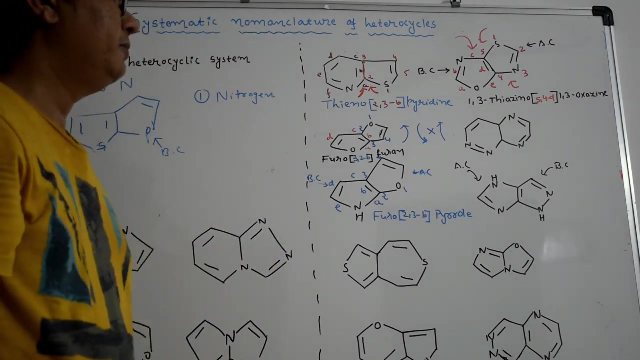 So lowest locate number are this: So your this ring is base component and this ring will become attached component Right, So so that a tribal name for this is possible. Right, A tribal name for this molecule is already given. So whenever the tribal names are there, we will use the tribal name. 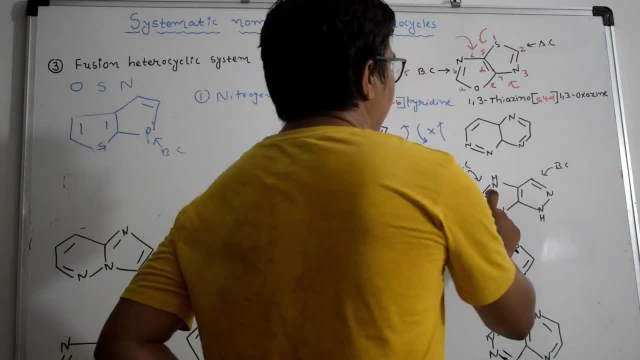 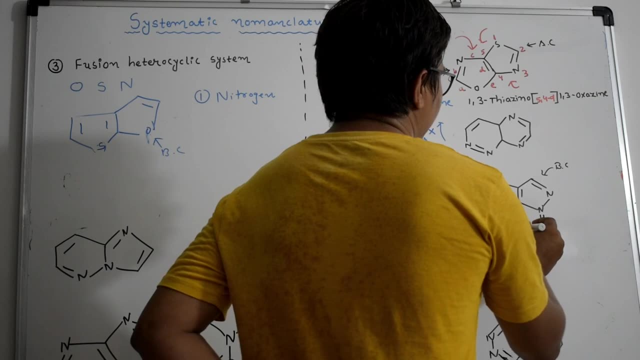 So this molecule is called as a pyrazote and this is called as a imidazote And attached component. so first I have to write attached component. So it will imidazote, square bracket right. and this is your pyrazote. 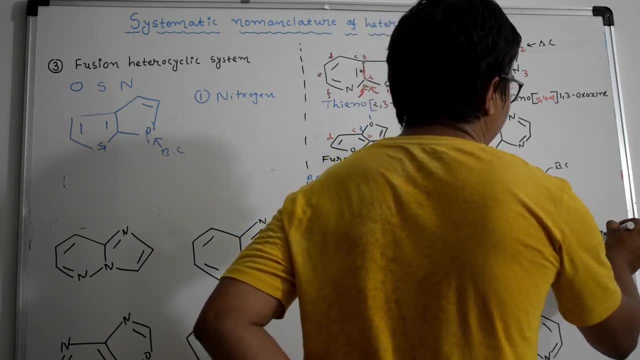 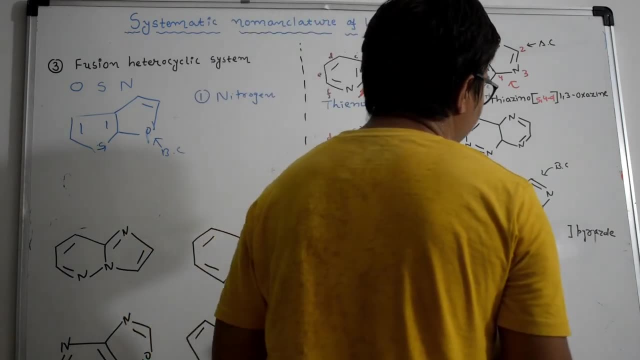 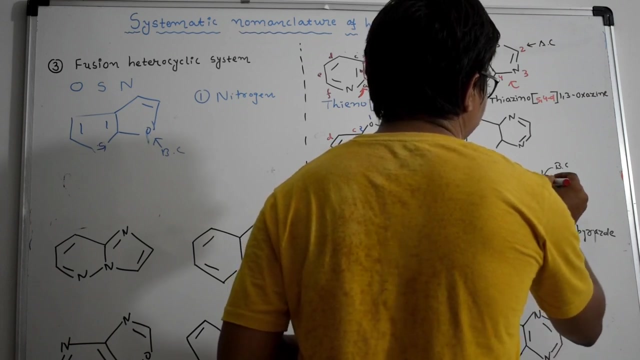 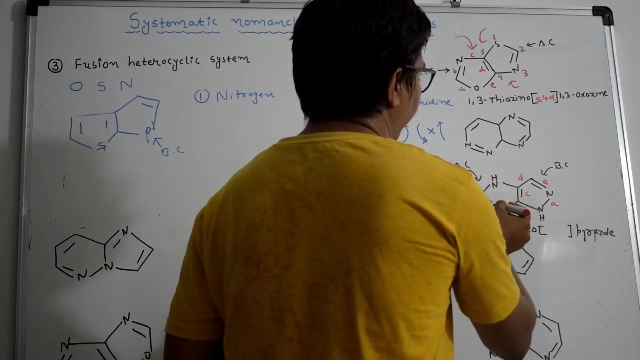 Now I have to give the alphabets to the, your base component. so your alphabets will goes like this right: A, B, C, D and E, and your- this is your attached component, where I have to use the numbering. 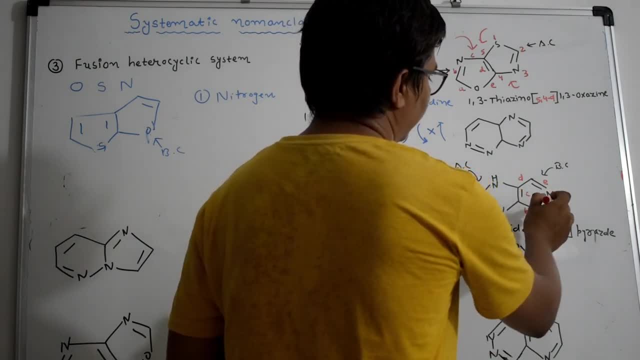 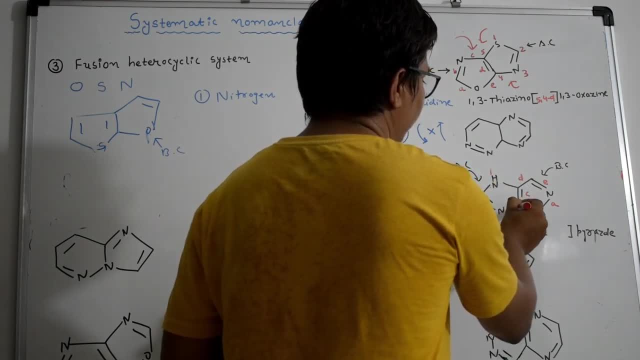 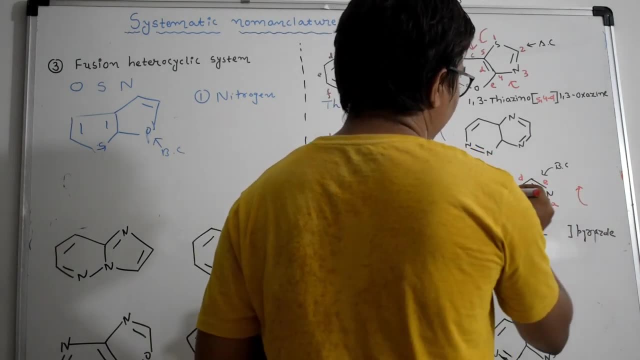 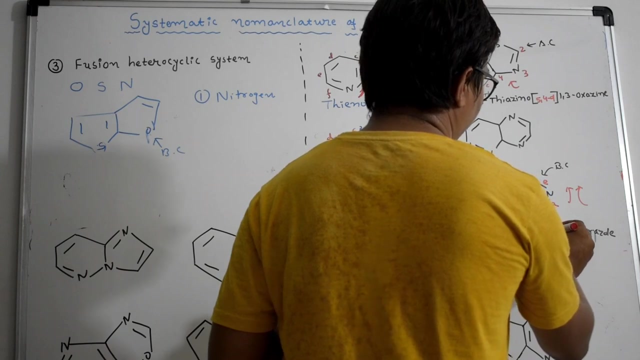 same direction, So 1,, 2,, 3,, 4 and 5, so your alphabetical order is going A, B, C, so in this direction, your numbering is also going into same direction, so it will become 4,, 5, C, right, imidazote. 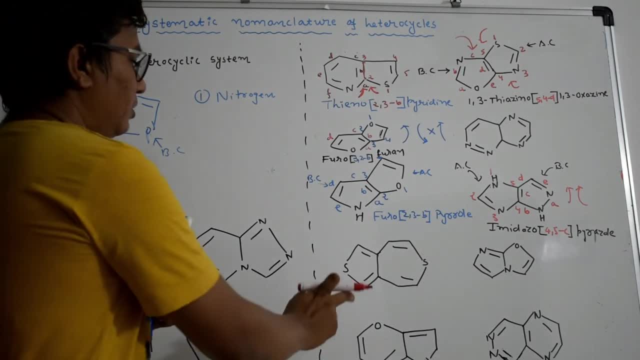 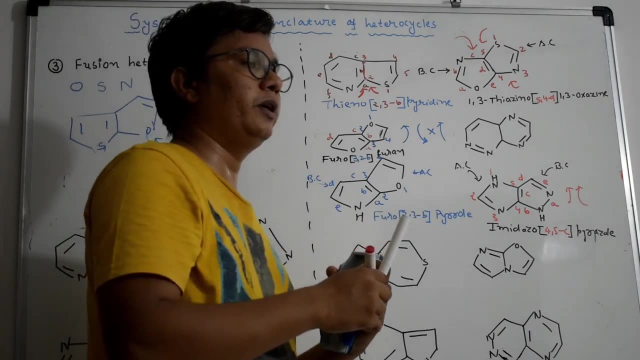 4,, 5, C pyrazote. Now let us come into the this example. here you can see the both. the cycle is contains sulfur as a heteroatom, but here the one is largest ring, 7-numbered, and one is a 5-numbered ring. 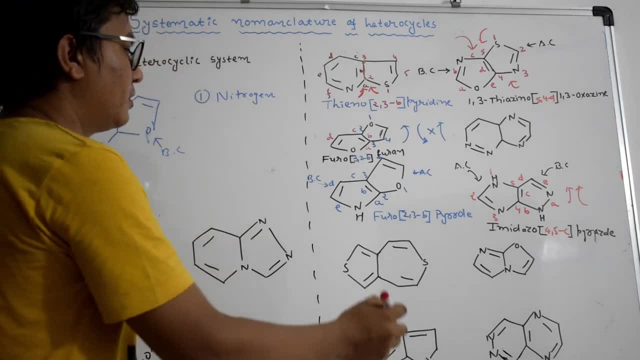 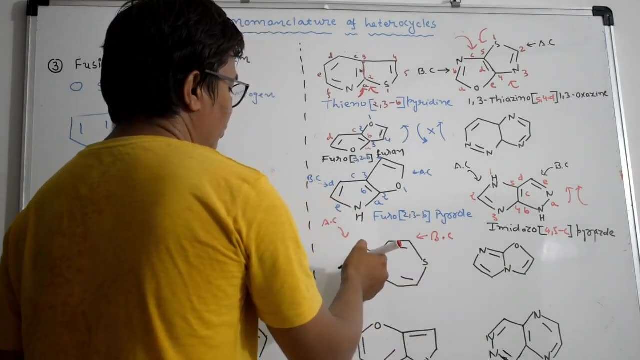 So 5-numbered ring. the bigger ring will be called as the base component. So here your: this ring is base component, right, and this ring is attached component. So the name of this ring is right: thiophene. so for the thiophene we will write thi-eno. 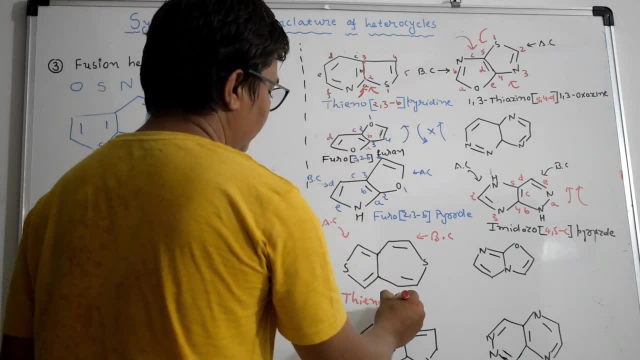 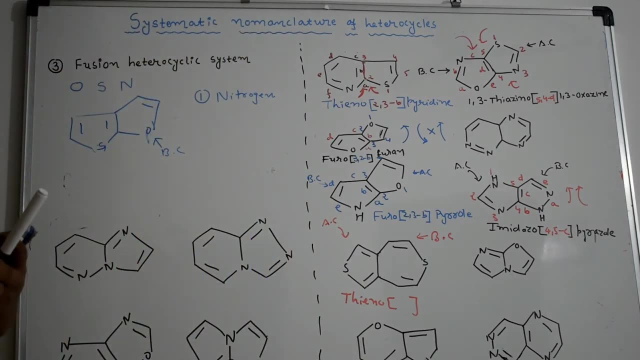 right. And for the 7-numbered ring the private name is not available so we have to give the systematic Hans Wittmann name to this molecule. so it is a 7-numbered ring. so I had we had discussed in the previous video that 7-numbered ring is that? so it will be called ap right. and 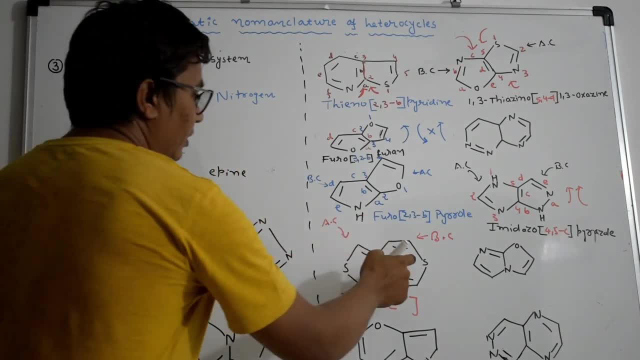 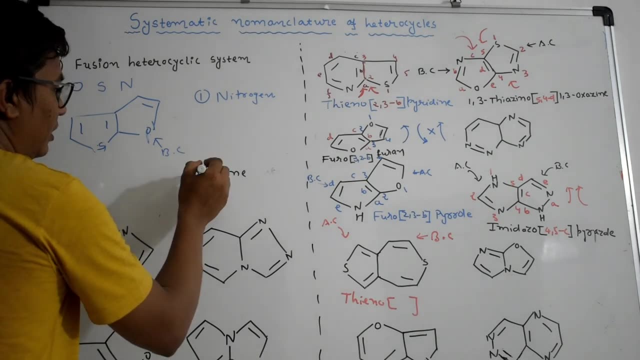 it is unsaturated, so it will be called apine, and the sulfur as a heteroatom, so it will be called thi-pine, right? So this is the 7-numbered ring. So here we have to drop the your vowel, because it is followed by the vowel, so it is a thi-pine. 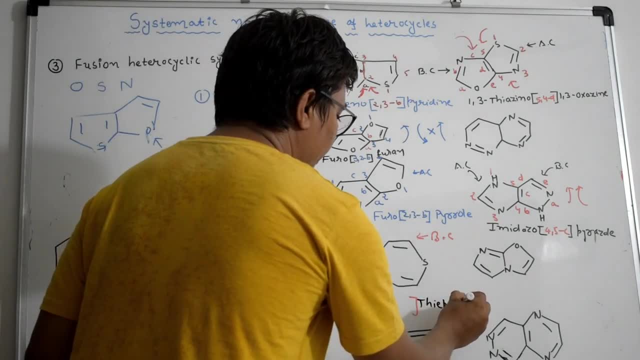 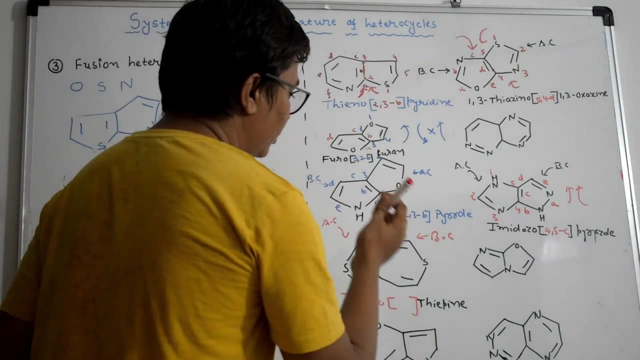 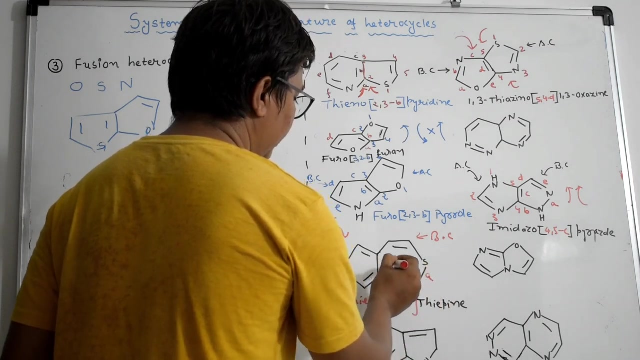 So I will write thi-pine. Now it is time to give the numbers. So for the base component, what I will do, I will go in like this direction: a, b, c, d, e and f. And for the same number, I will write a, b, c, d, e and f. 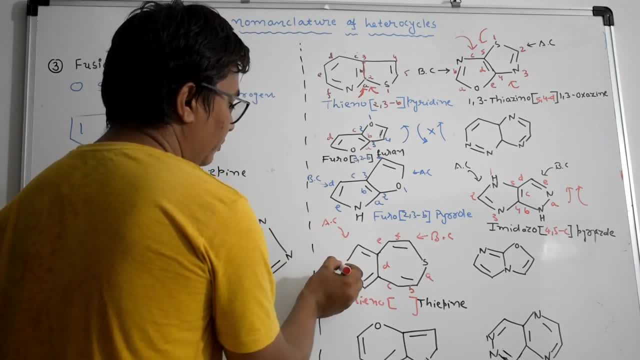 And for the same number I will write a, b, c, d, e and f, And for the same, to attach the component, I have to give a numbering 1,, 2,, 3,, 4, right. 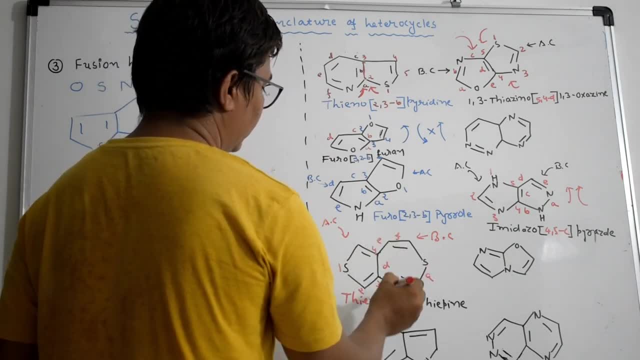 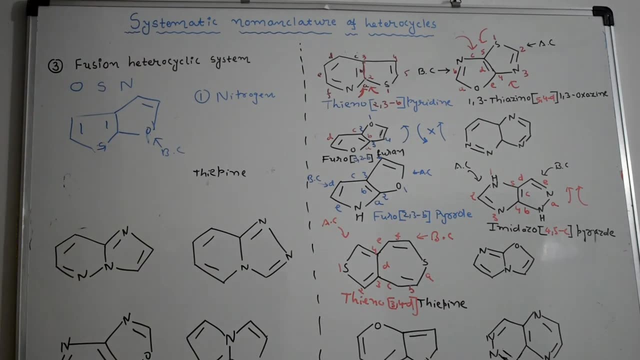 So this is in this direction. this is also going to this same direction. it will be 3, 4, d thi-pine, right 3, 4, d thi-pine. Now let us come on to this example. 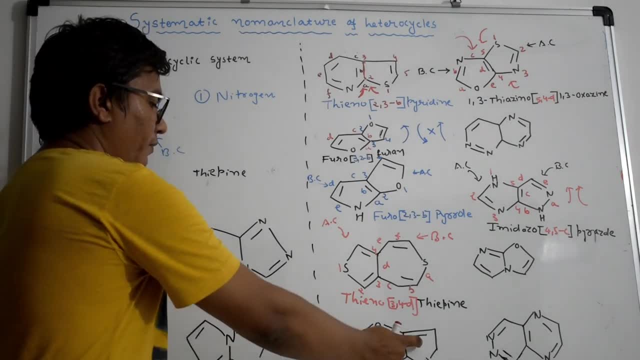 So here in this example, one is the 6-numbered ring, one is the 5-numbered ring, and both of them contain oxygen atoms. So the bigger the or the larger the ring, it will be the 5-numbered ring and both of. 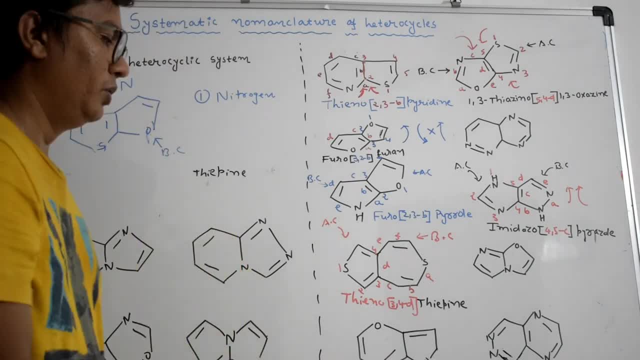 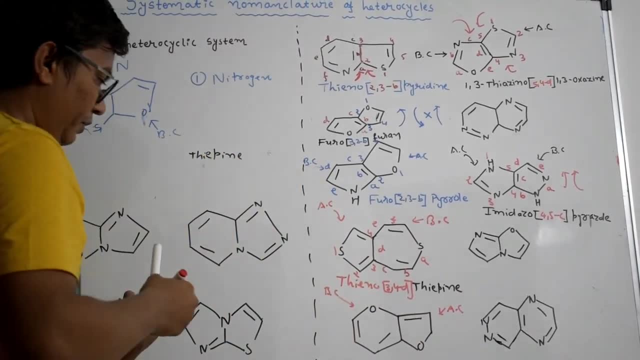 them contain oxygen atoms And it will be called as the base component. So here, this ring is a base component and this ring is a attached component. So what I will do now? I will start with the name of attached component. it's a furon. 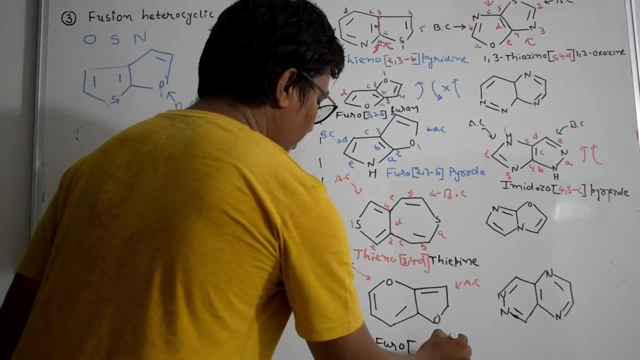 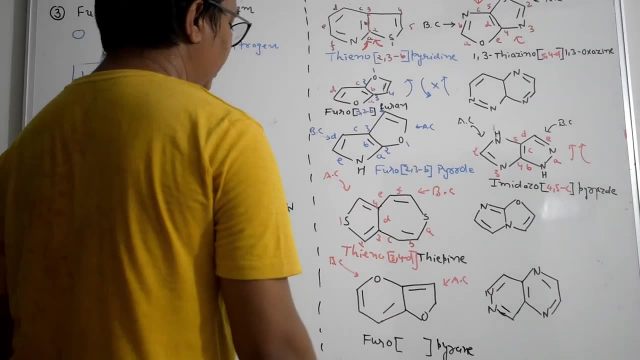 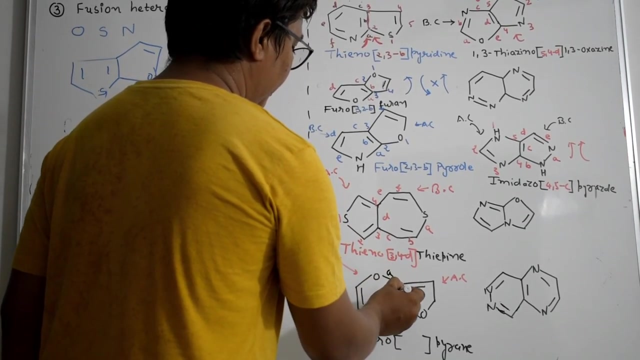 so furon, we will write furo and it's a 6-numbered ring oxygen, so it is called the pyrane. So I will give the alphabets to the base component first. So the alphabet I can get like A, B, C, D and E and if I will give the numbering from, 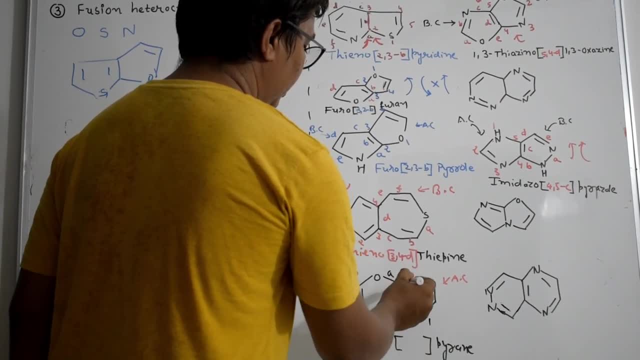 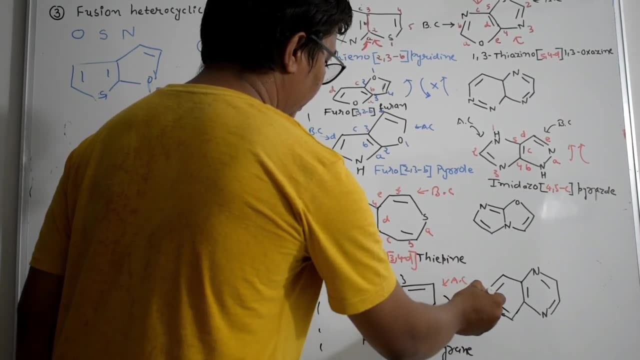 here it's a 1,, 2,, 3, so your A, B, C is going to this direction and your numbering going to this direction. It will not work, so I have to take the numbering from this direction. 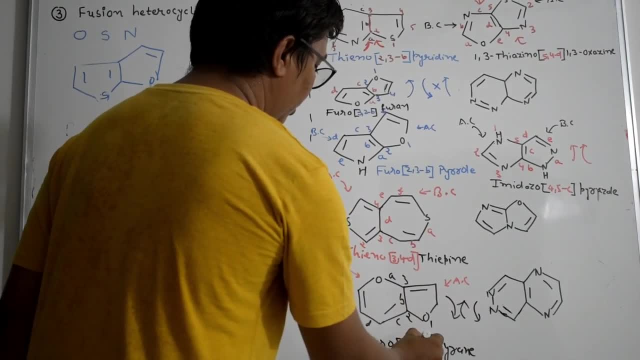 So from this direction, 3 will come first. So 3,, 2, B pyrane. Let's come on to the another example. Let's take the numbering from this direction. So from this direction, 3 will come first. 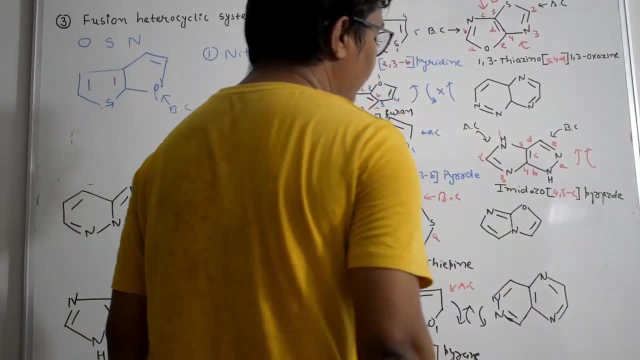 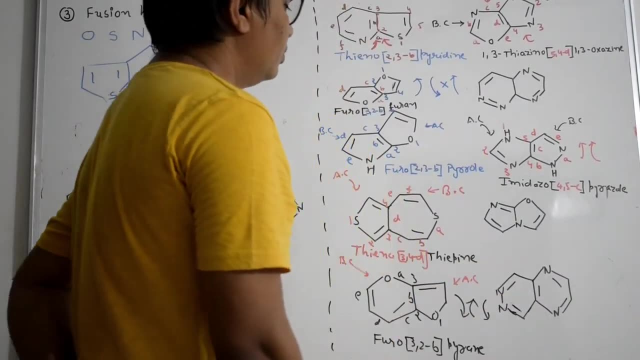 So 3,, 2, B, pyrane, Let's take this example. So here, in this example, what is the 6-numbered and what contains the nitrogen? So what I have to do, I have to take the lowest locate number. 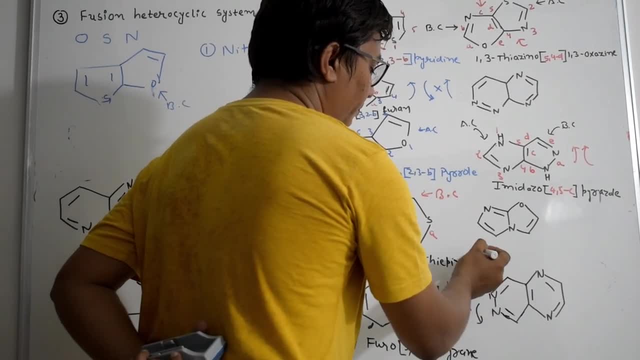 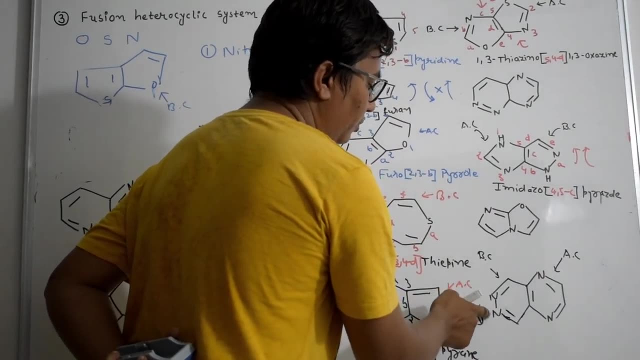 Here 1, 4 position to each other and here 1, 2,. so this will become your base component and this will become your attached component. Again, I will tell you, because these are near to each other: 1, 2, and here 1, 4.. 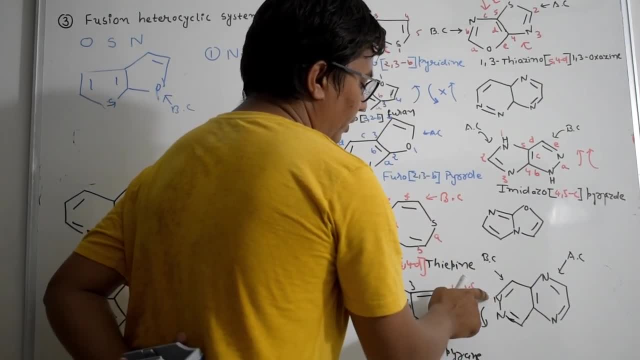 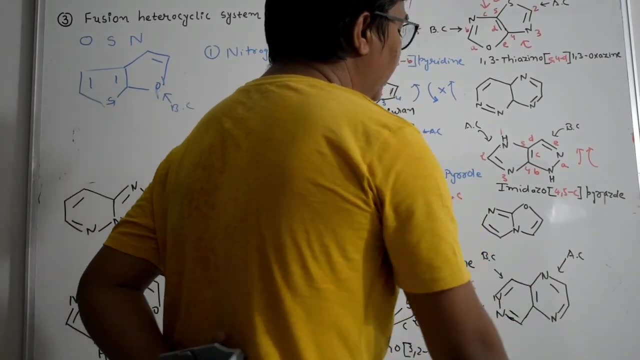 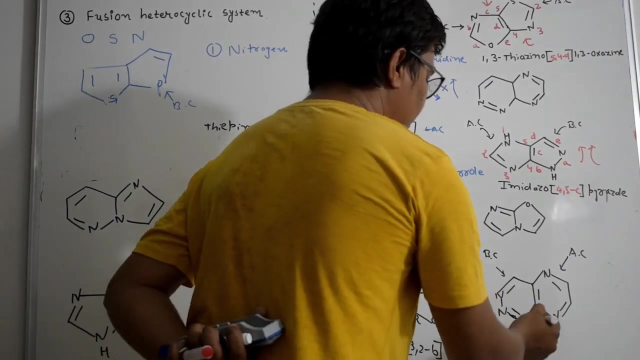 So whenever this kind of situations are there, So that 2 heteroatoms near to each other will be called as the base component, So attached component and this ring, for both the ring tribal name is there For 1,, 4 position, it will be called as your pyrazine ring. 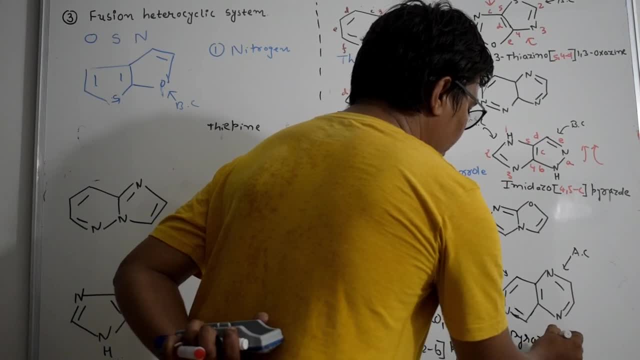 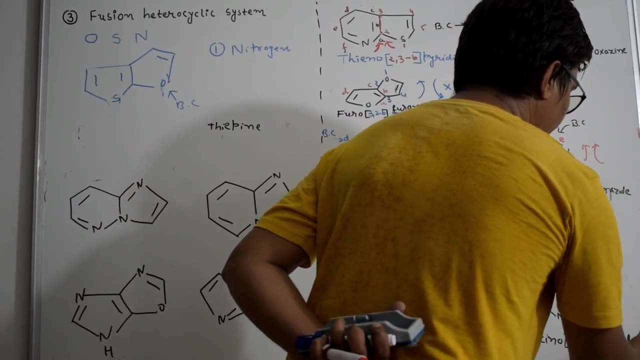 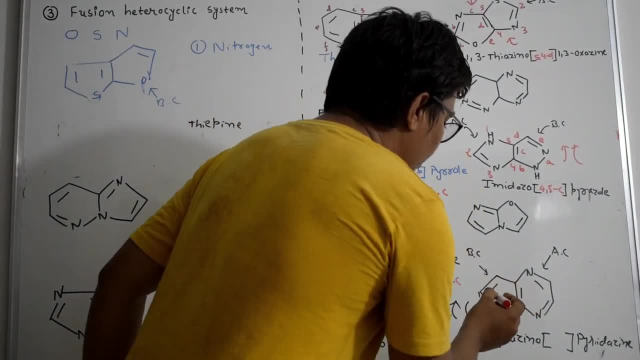 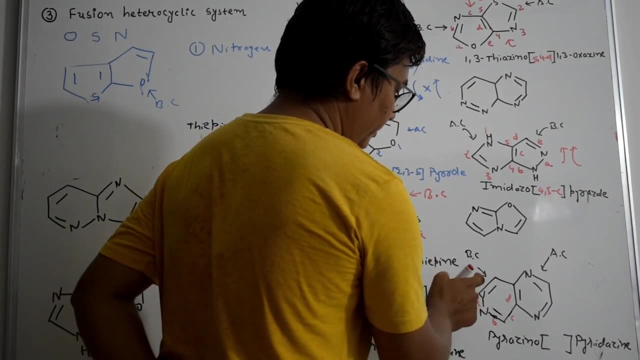 And now we have the numbering and the alpha critical order. So this is the heteroatom. I will call A, B C D. If I will go on this reaction, A B C D, so on both the directions this bond is getting D number. 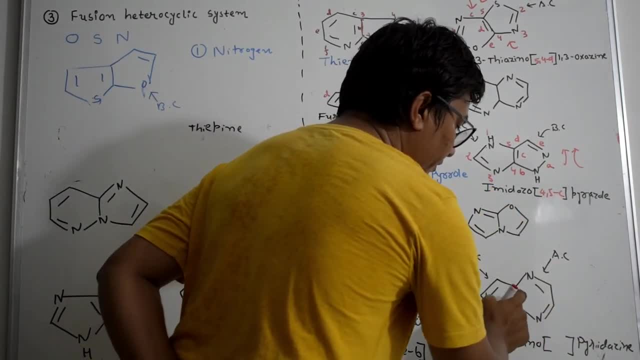 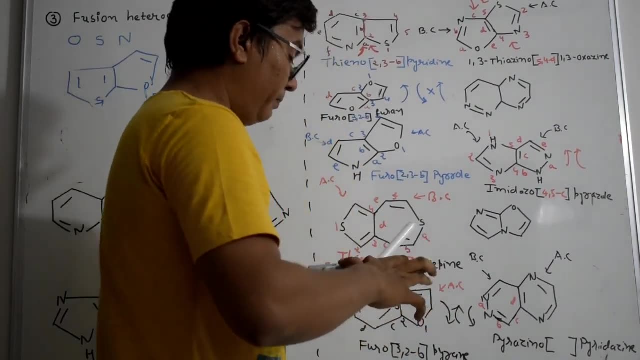 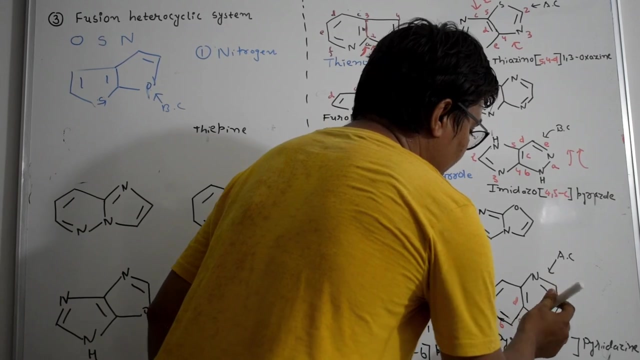 So, according to numbering on the second ring, we will give the numbering on this direction or this direction. Let's see, We will try to bring both of them, bring both the direction of the same. So if I will start from here, it will be 1,, 2,, 3,, 4.. 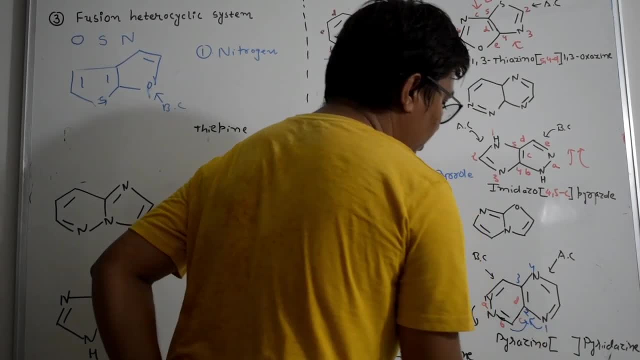 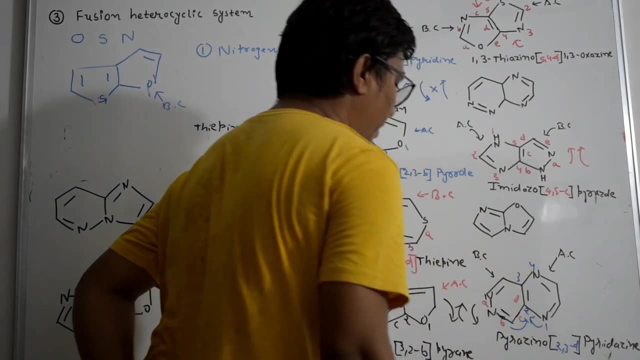 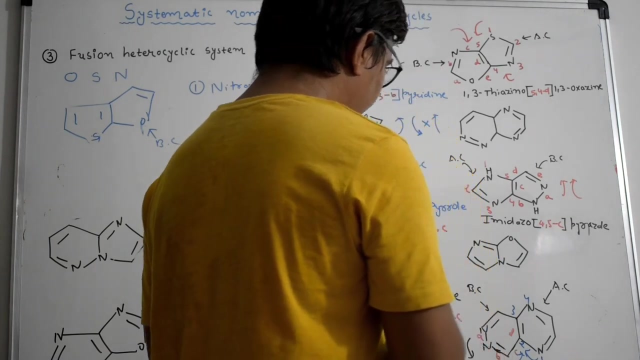 So it is going into this direction. the same way, this is going into this direction, So I will write 2, 3, d, So pi d is you know, 2, 3, d, pi d, d. Now let us see this example. For this example, 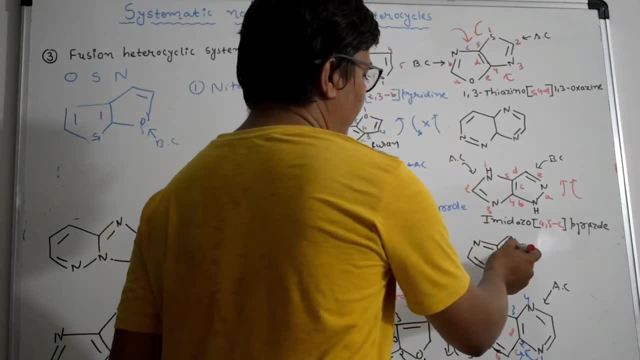 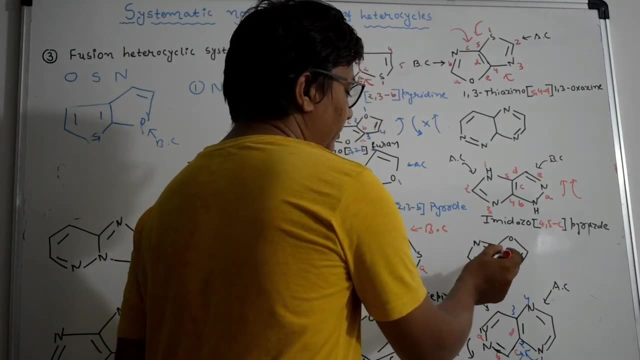 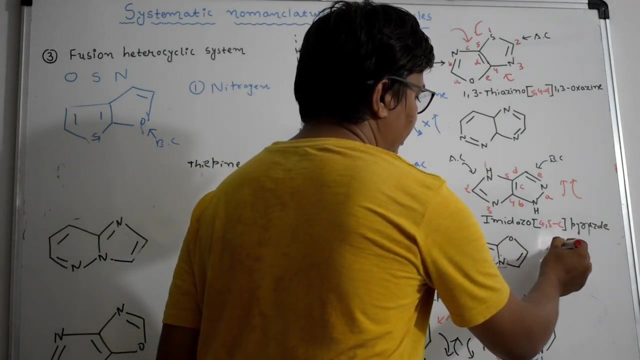 you can see, both the rings are 5-membered rings and the nitrogen atom at the junction of the two rings. So this nitrogen atom will be considered as a part of both the rings, right? So here, if you will just divide both the rings, then this nitrogen atom will be considered as a part of. 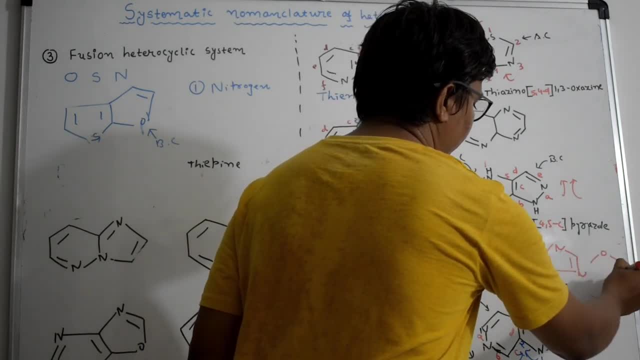 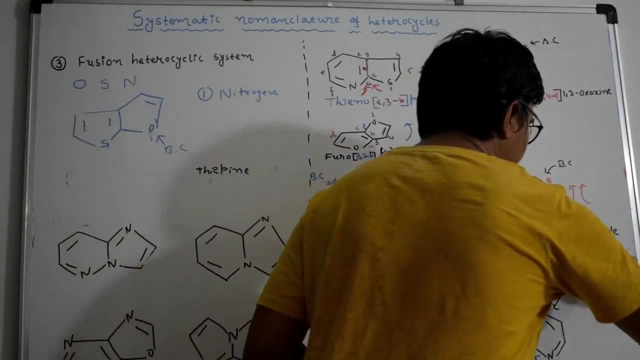 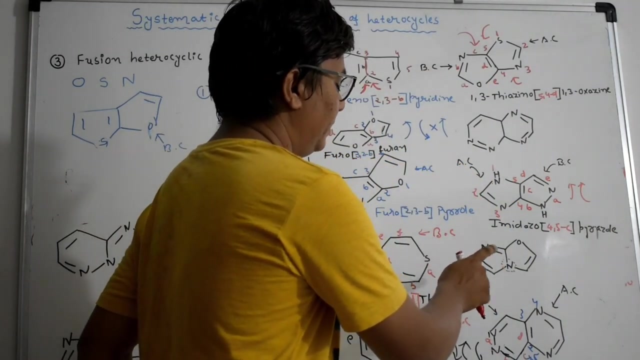 both the rings. So this is your first ring and this is your second ring. like this way, It is part of both the rings. Now how we will give the nomenclature to this molecule. So first we have to decide the base component. So here oxygen and nitrogen, here nitrogen and nitrogen are there. In that case, 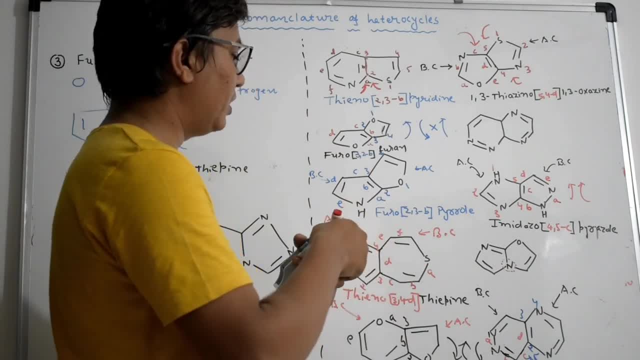 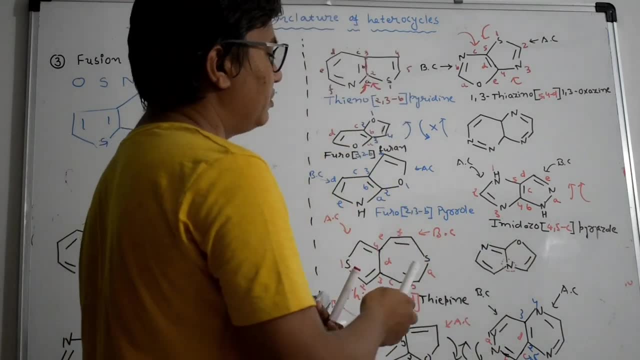 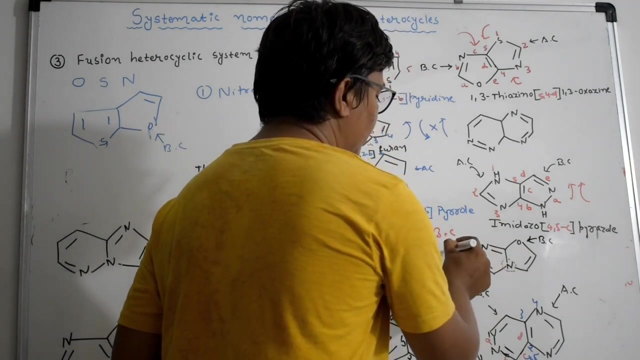 what we have to do, the ring which have the variety of hydroatoms- right Here there are two nitrogen and here there are oxygen and nitrogen, So variety of hydroatoms is present into this ring. So it will be called as the The base component And this will be called as the attached component. 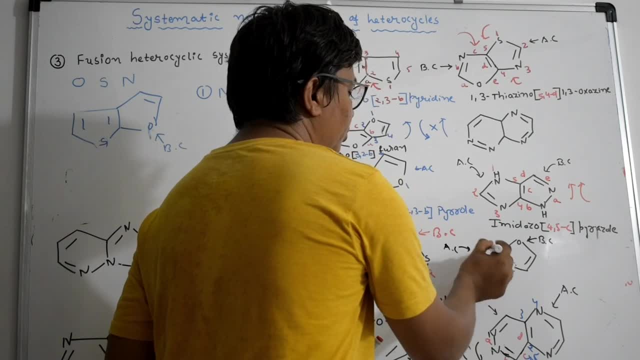 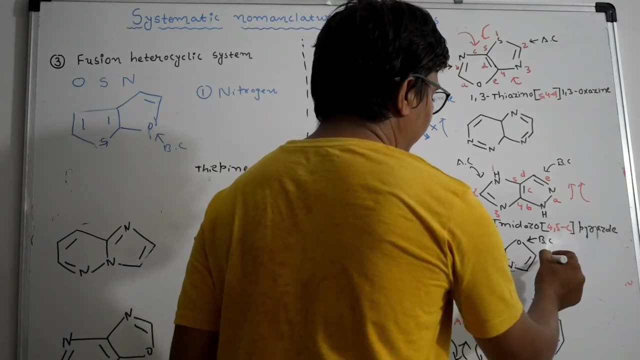 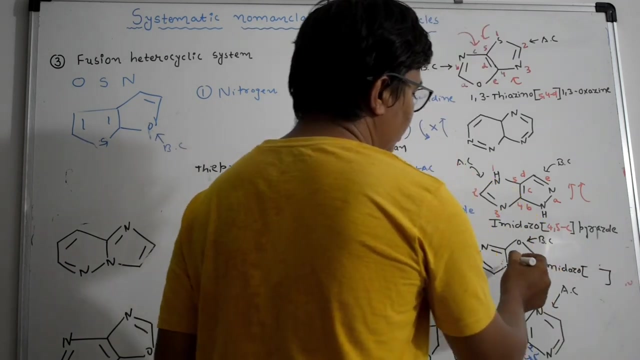 So attached component is on one-third position of each other. so for this molecule, as we know, the tribylane is present. as you have to write, like Imidazole, Imidazole in square bracket. This is your oxygen and nitrogen up to 1, 3rd position. 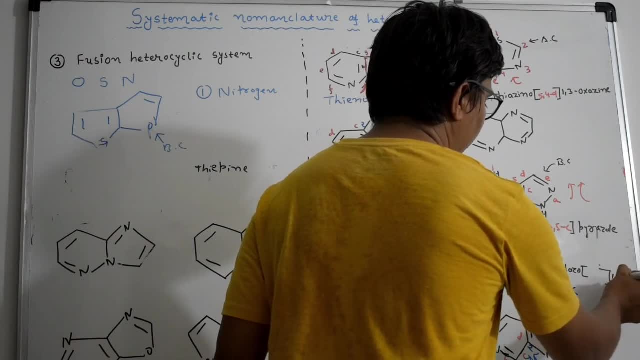 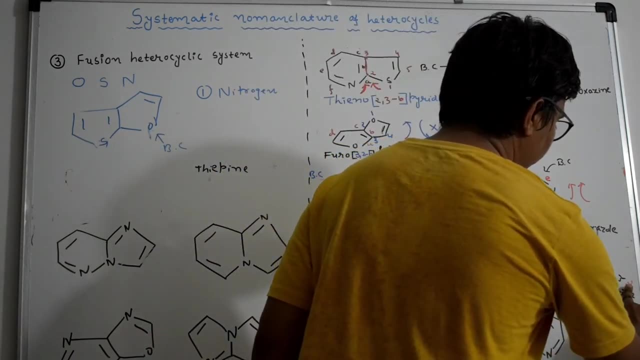 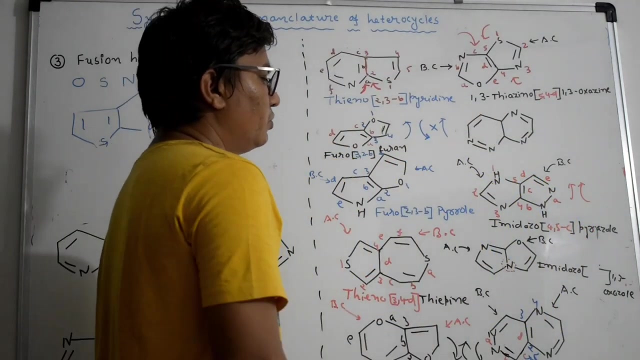 of each other. Oxygen comes first, So 1. third oxazine right. one third oxazine. now it's a five membered ring, so i will call it oxazole, oxazole. if it is a sex membered ring, then it will be oxazine. so imidazole, one. three oxazole: now i 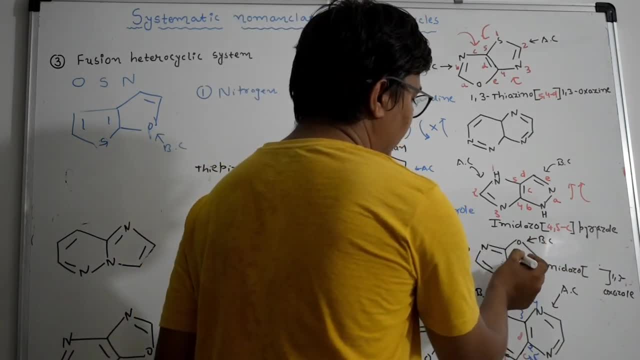 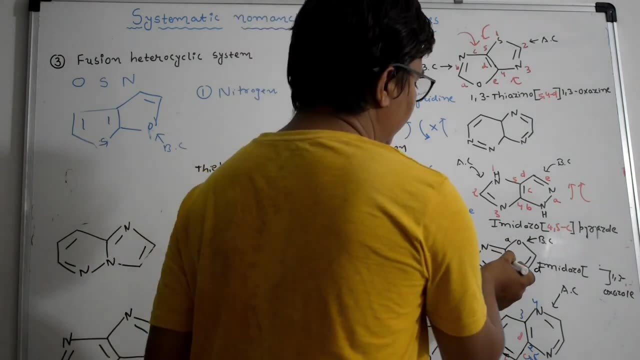 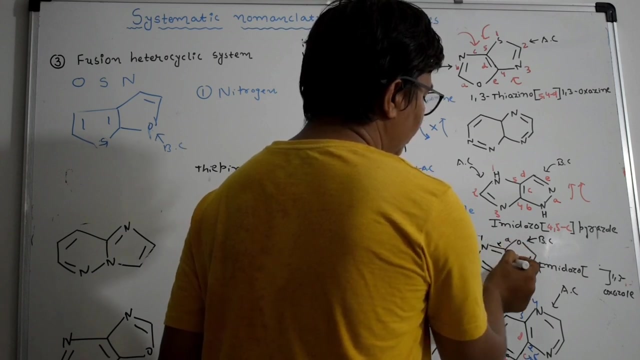 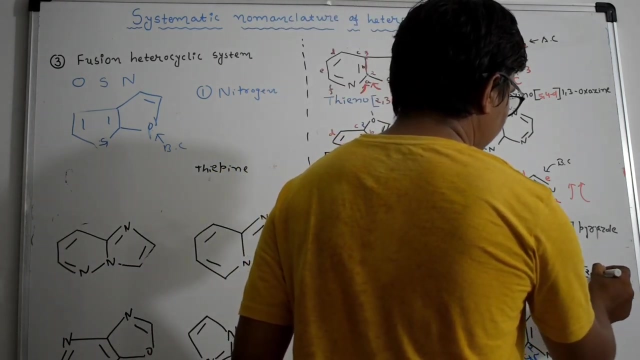 have to give you numbering. this is your base component. so start from where? from the oxygen, a, b, c, d, right from here we will go from this number so it will be called your one, two, three, four, right. so it is two, three, b, one, three, oxazole. now let us come on to this example. 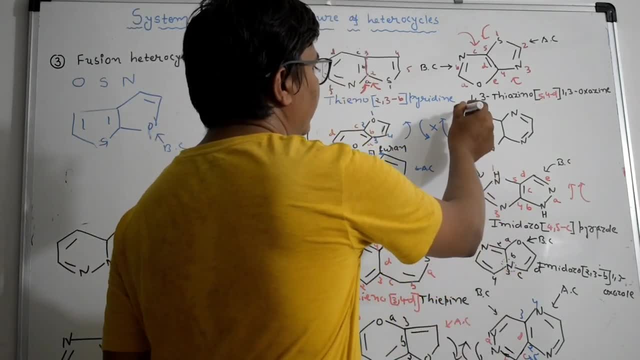 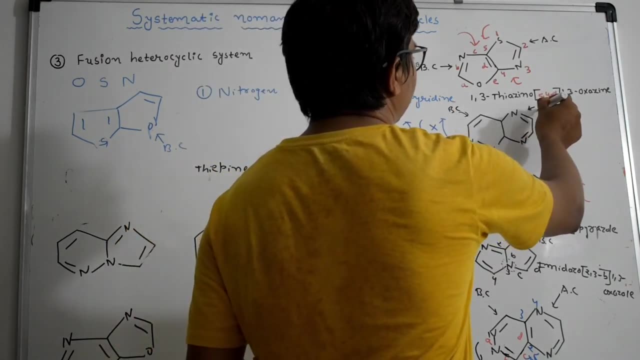 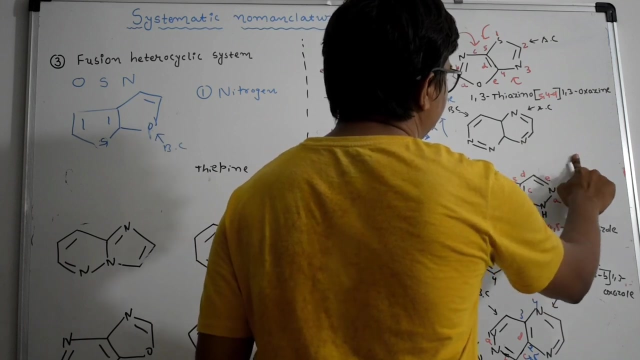 there are two ring. the lowest located ring will be called as base component. so this is the base component. we already have seen this. for example, like this: and this is your attached component. so first i will write the attached component. it is your pyrazine. for the pyrazine, we will write pyrazino and 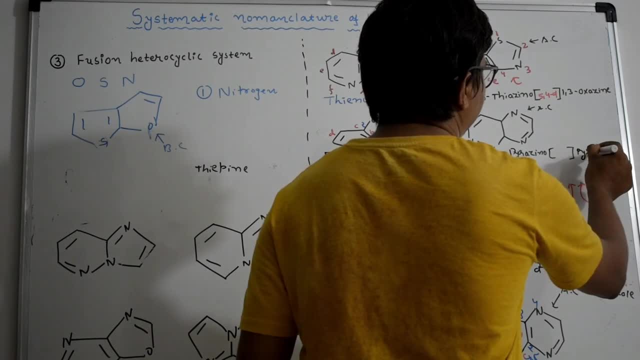 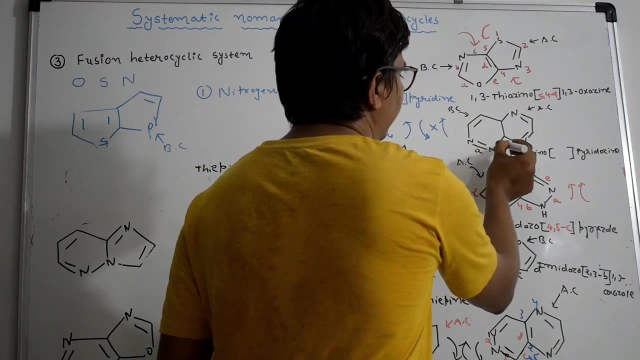 this is your pyrydazine ring. this is your base component. sorry if the data ring from A to Zome, from A to Zome, So it is может be Bvee of sir, Bvee of sir Celle, Celle, as Dogon of sirll said So. 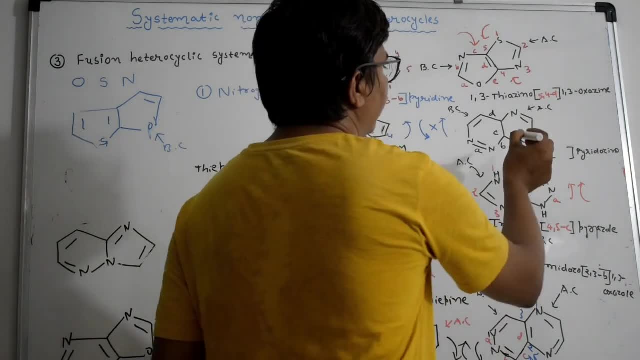 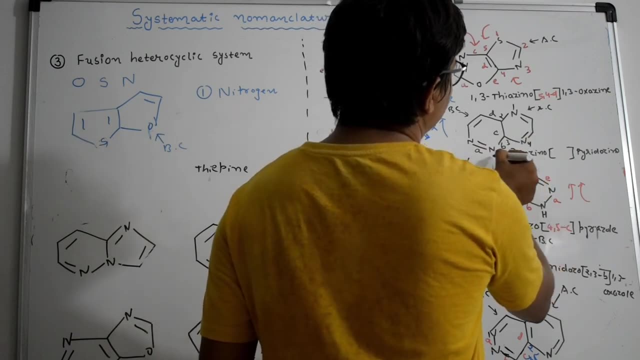 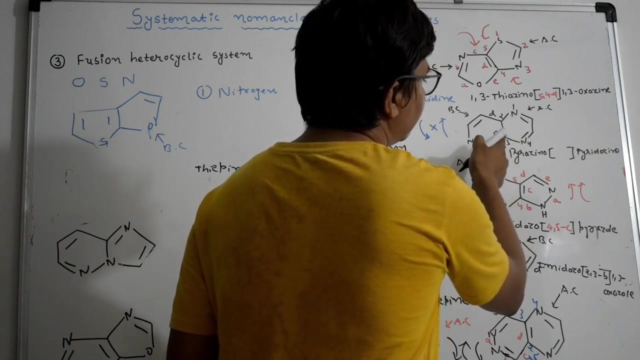 A, B, C, D, and here I will give the numbering from 1,, 2,, 3,, 4, so it is going in this direction. Now you can see, here the numbering from the border side is possible and it gave the same. 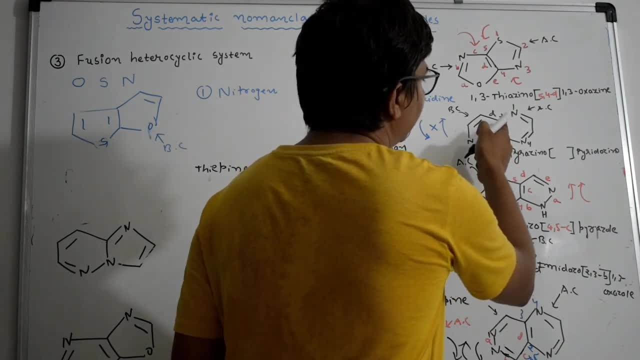 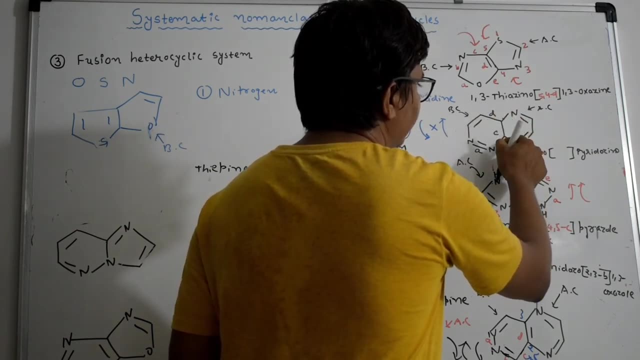 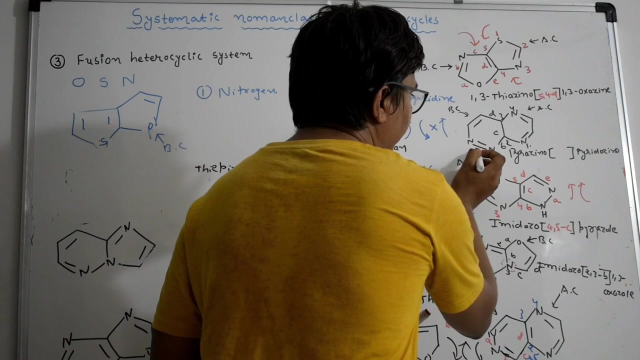 number. but if I will go like this, it will give the 3, 2 position. So instead of giving the numbering from this side, I have to give the number from this side right: 1, 2, 3, 4,. hope you are understanding what I want to say. I have to give the lettering. 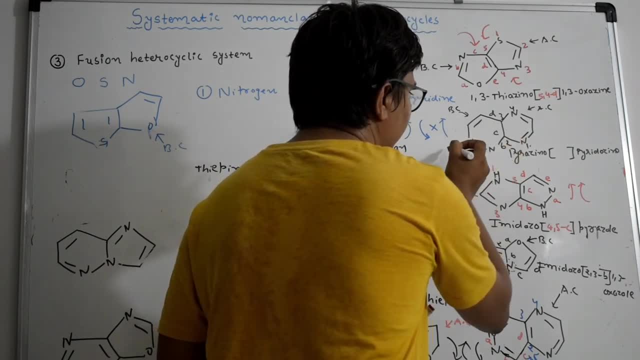 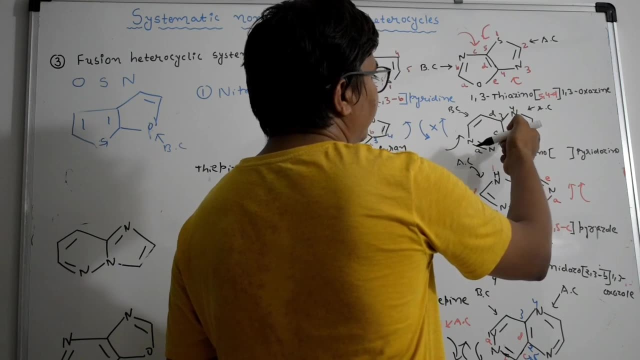 from the alphabet from this side: A, B, C, D. so it is going this. If I will do the numbering from this side: 1,, 2,, 3,, 4, right, so it will come in which. 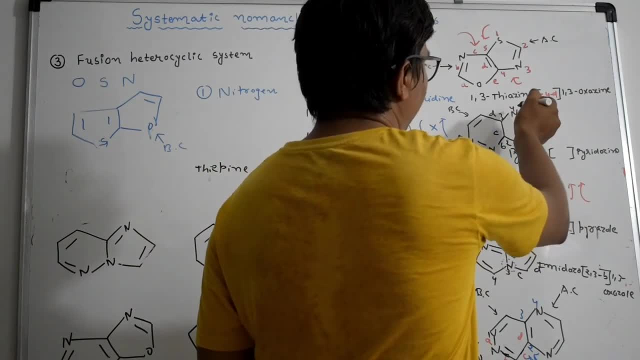 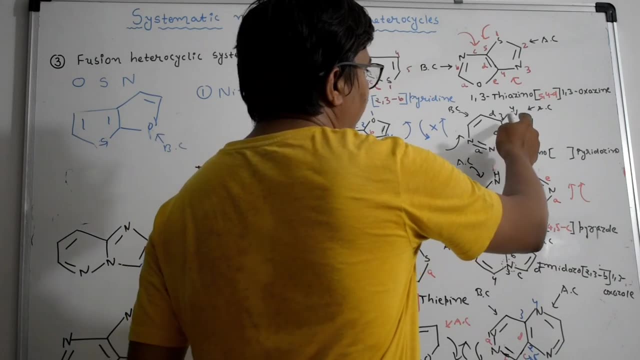 order. it will come into the your opposite order. it will come like opposite. so you have to take the numbering from this side. so it will come 3, 2.. So instead of giving the numbering from this side, we have to give the this side, so we 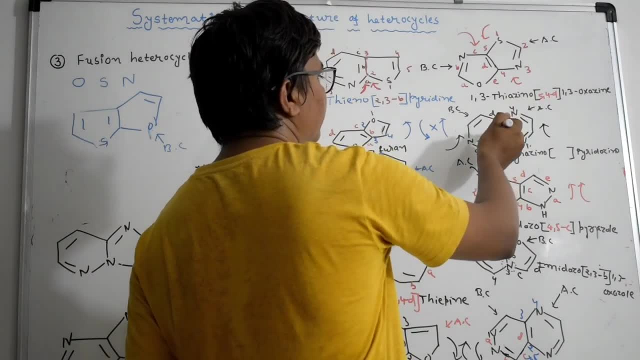 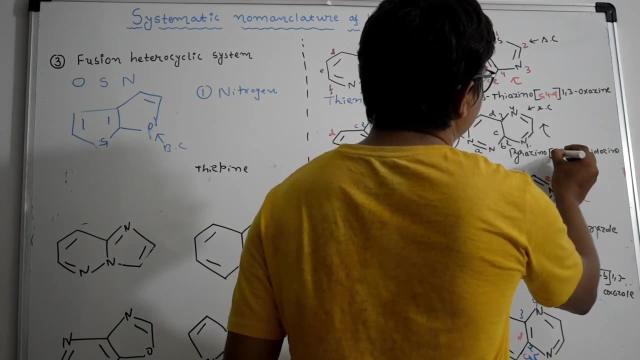 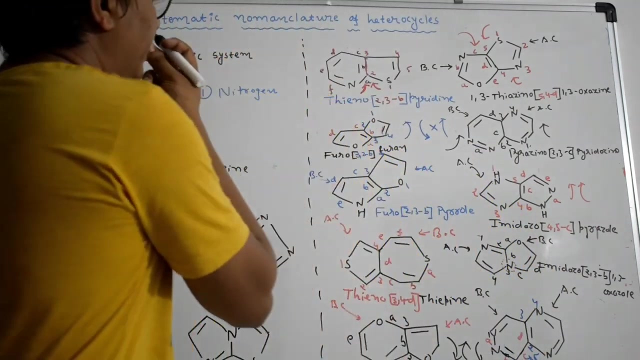 do not have to change anything because numbering will remain same whether you will start from this or from this side. So here is 2,, 3, right, and it is on to C, A, B and C. so pi raised to 0,, 2,, 3,, C pi. 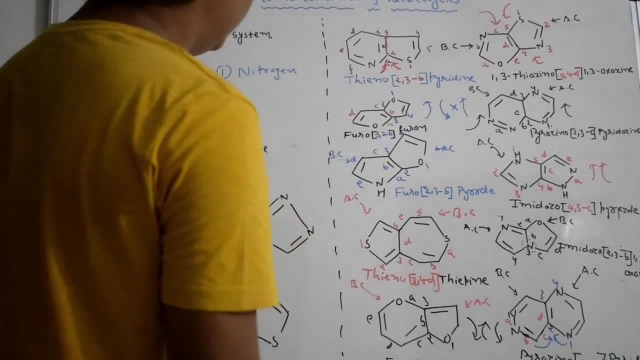 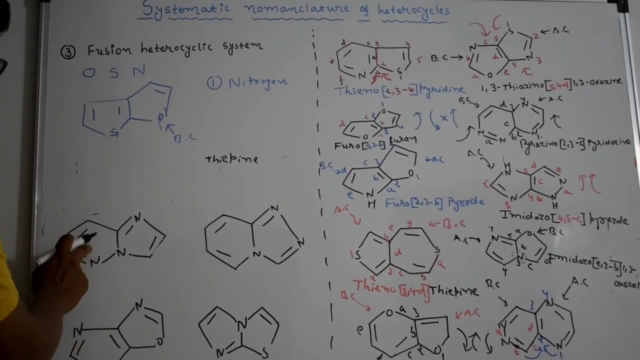 raised to 0, right, So we had finished on this side, let us come on here. So here again, 1 is a 6-membered ring. 1 is a 5-membered ring. the bigger ring or largest ring will be called as a base component. 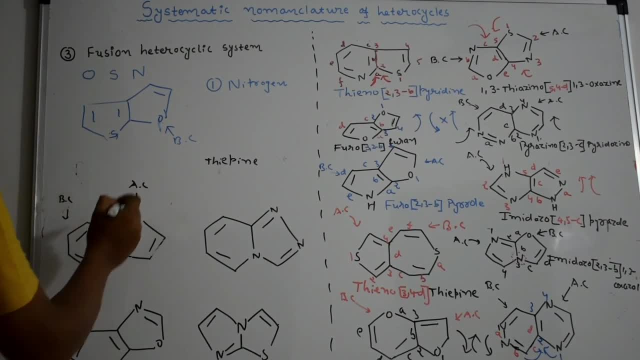 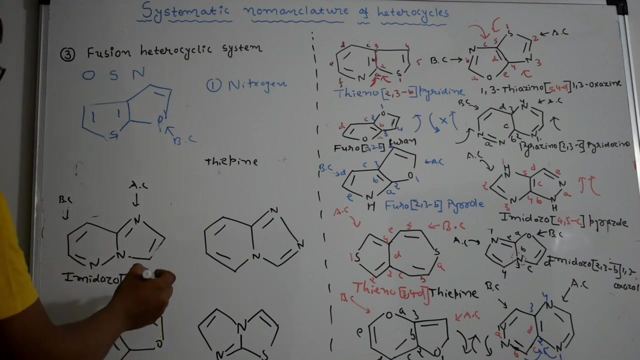 Here is your base component. here is your attached component. So attached component is a one-third position, so it is called imidazo And this is nitrogen ring adjacent to each other, so it will called your pyridazine. it is called pyridazine. 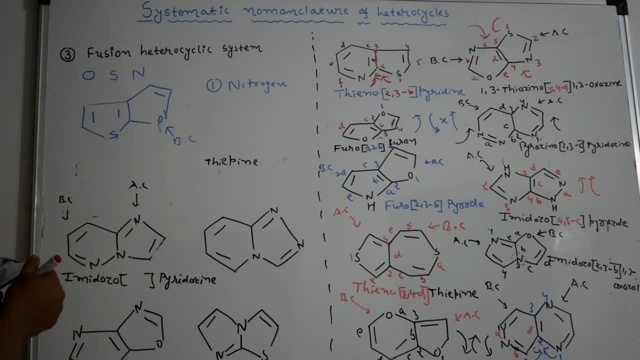 Now to base component. what I have to do here. the alphabets A, B, C, D and from the attached component I will go on this direction. it will take the numbering from here: 1,, 2,. 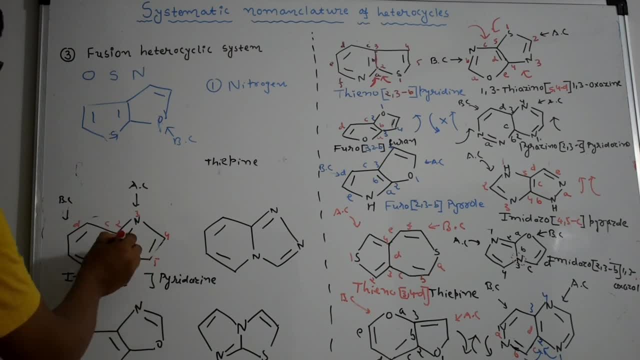 3, 4, 5, because whether I will start from this or this, so it will have a your, your numbering will be 1, 2, B right. 1, 2, B pyridazine. 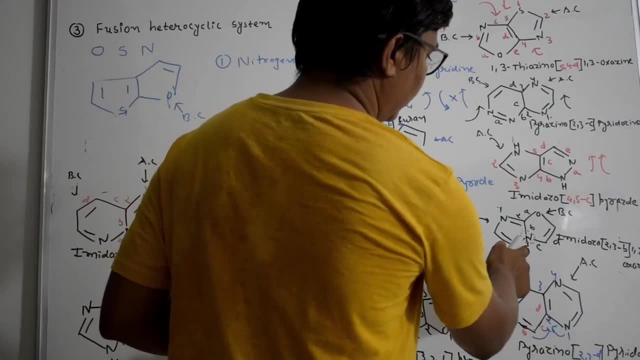 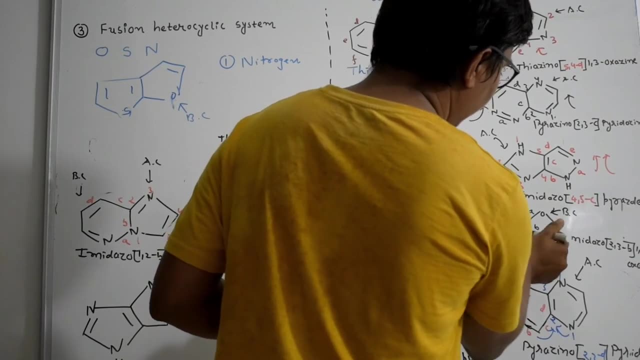 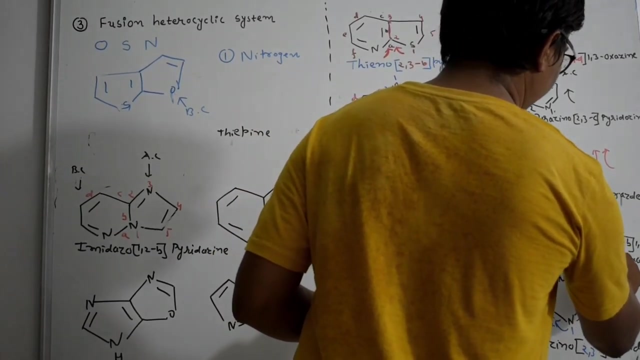 Here we had made the one mistake right. So here is the atom, is there? so what we will do: 1, 2, 3, instead of 1, 2, 3,. I can go like this: 1, 2, 3, so that there is a little correction. so I will have right, it is 1,. 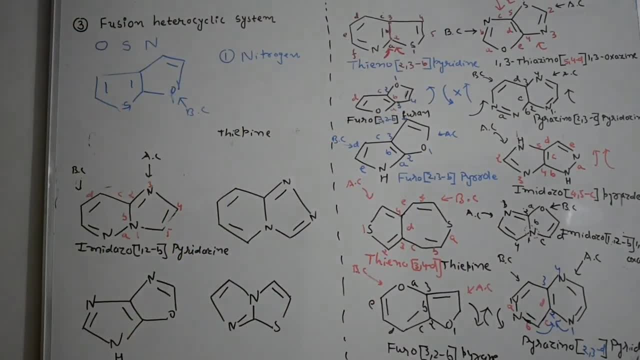 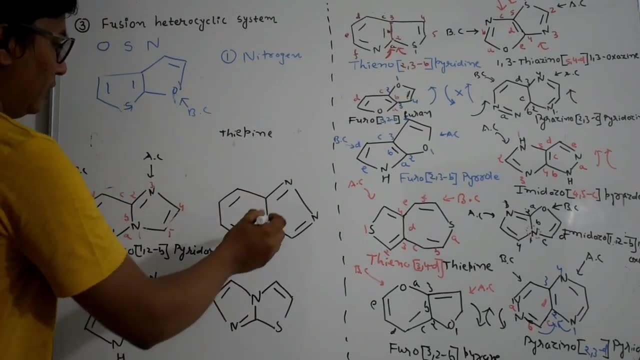 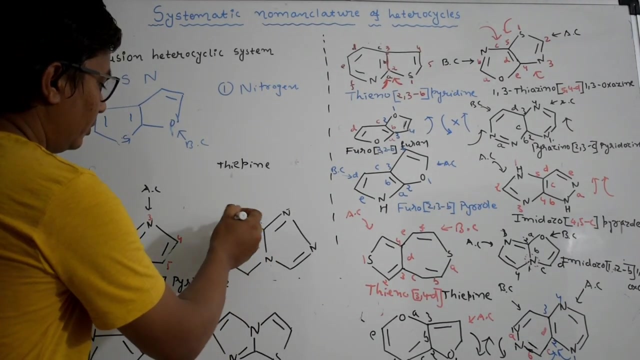 2. Let's come to the this example. So this is your base component and this is your attached component. See, for this molecule, your, this bigger number ring will be your largest ring, will be called as your base component. this will be your attached component. 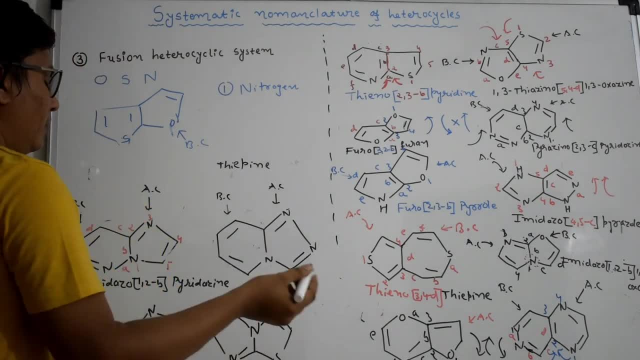 So in attached component we have to give it possible lowest numbering. so it will one, two, three, four. So your attached component, this will be the biggest numbering and this will be the largest numbering. So that is the overall numbering. 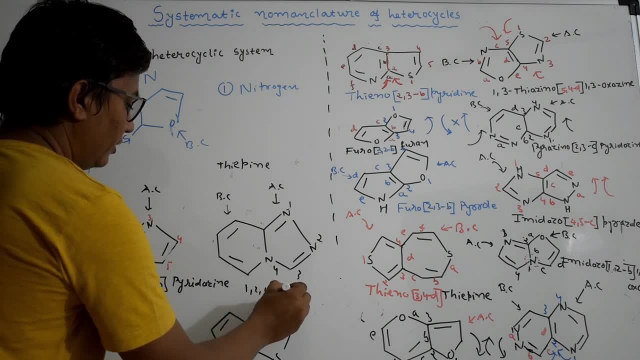 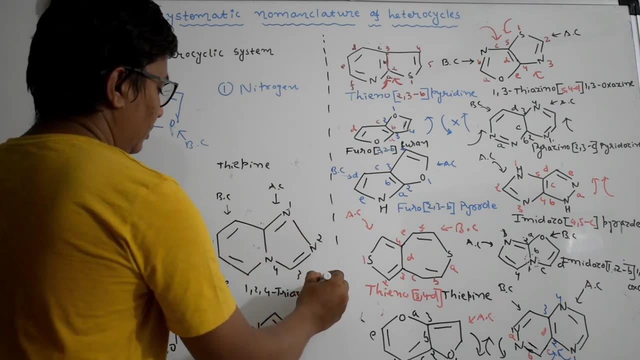 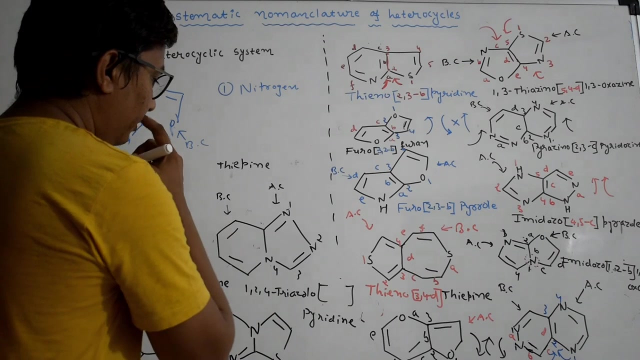 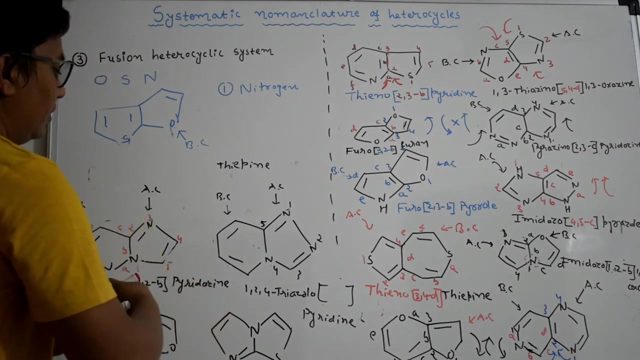 Okay, Okay, net is one, two, four, three, nitrogen. so try that as and the the fiber means it will try as a low square bracket and this is pirating. and I have given number one, two, three, four, five and your this alphabet will be go, a, B, C, D, like in this: 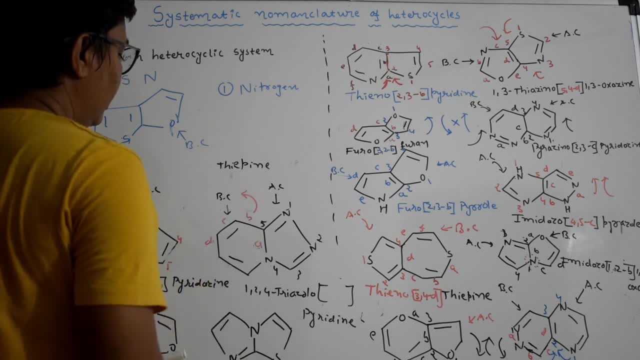 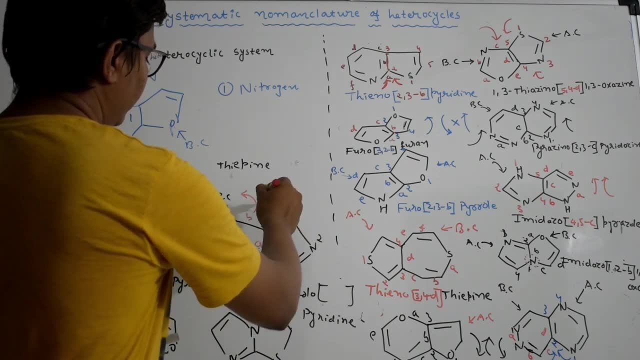 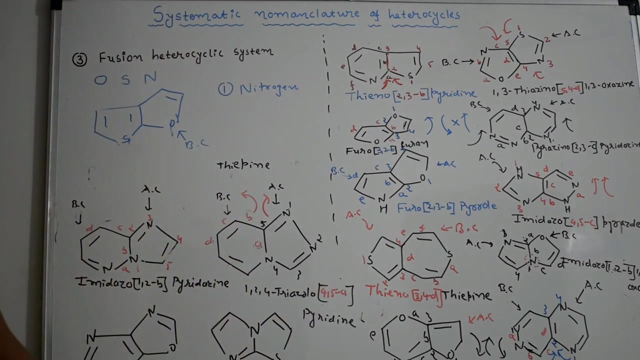 manner. so it is going ABC this way and here your numbering is going like in this way: four, five. so it will be called four five eight by reading. now let's come on to the this example. so here the two nitrogen term, nitrogen and sulfur, the variety of 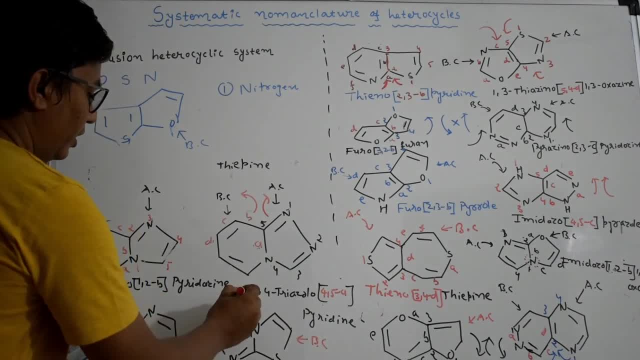 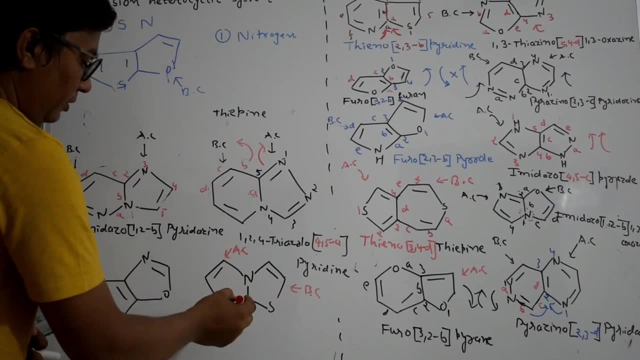 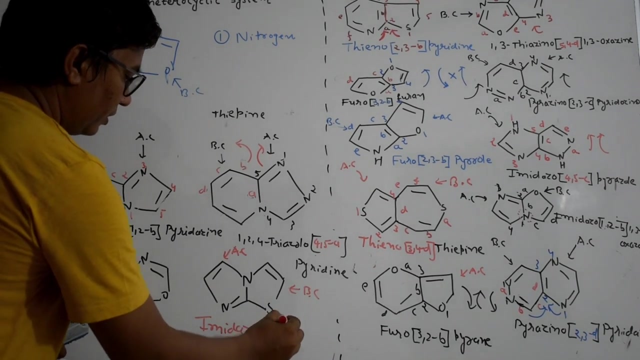 hyper atoms there. so this is your base component, this is your attached component. for the base component, we will give the alphabets and for the text component, the attached component is the one three position. so it will call imidazole and where we have to give the number imidazole, and this is your. 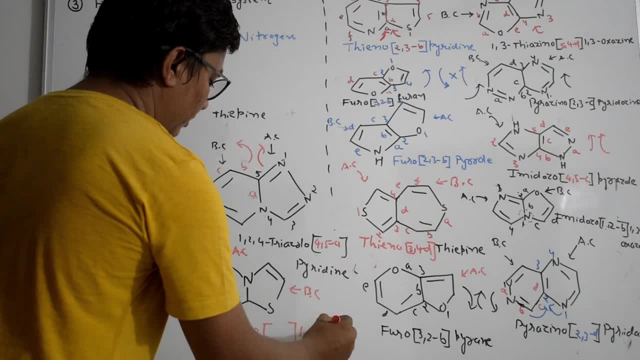 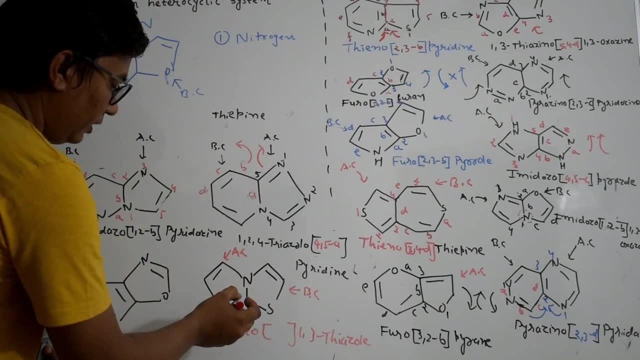 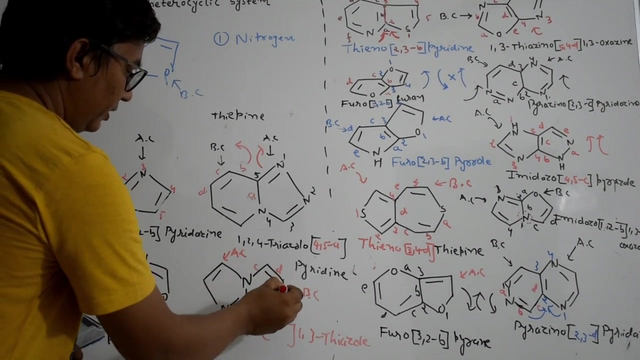 nitrogen and sulfur under the one three position. somewhere compressed it will called try as all. can I use this as the same thing? is it one 1990? let us give the alphabet to the base component a-b-c-d and he-and-訪 and he-and-訪. 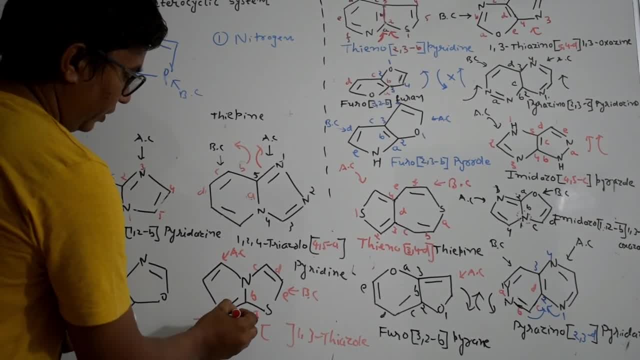 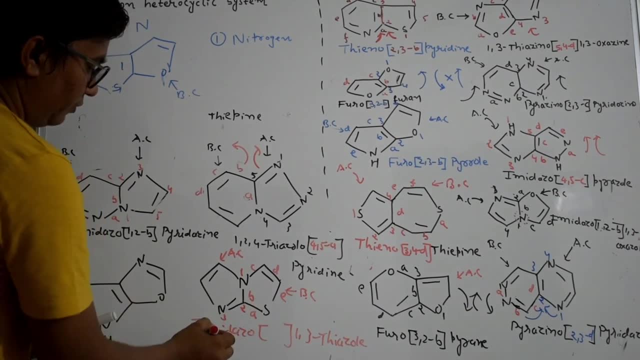 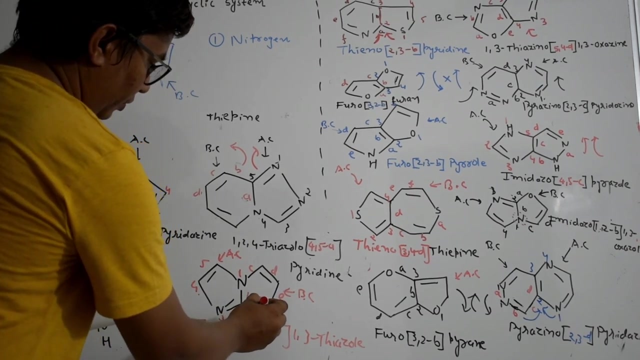 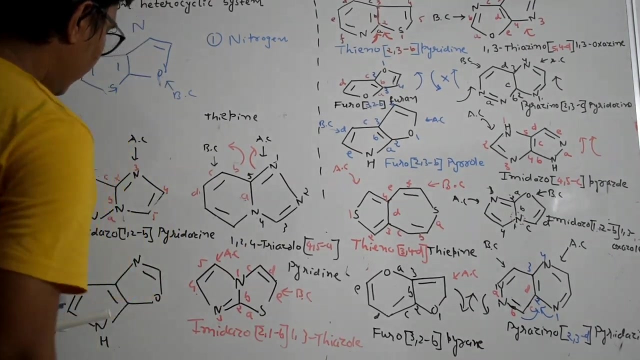 numbers. your numbers will be like one possible locals numbers. I can start from here: also 132, getting one number, 145. so it is your. this is going into this direction: ABC, and it's coming one. so I have to take two, one B. now let's come on to this example. this is your base component. 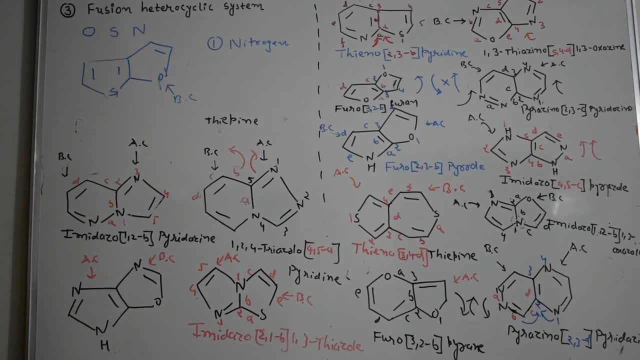 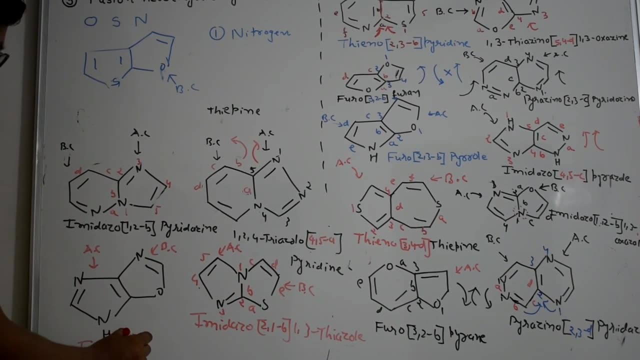 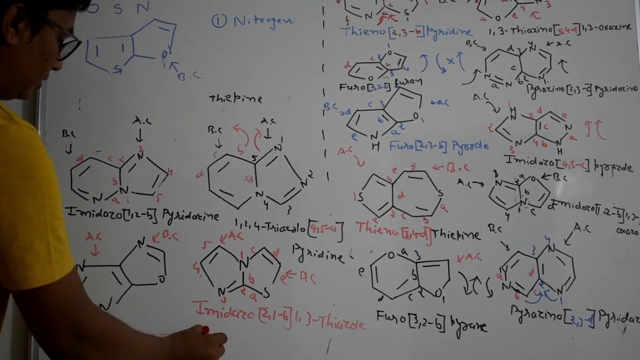 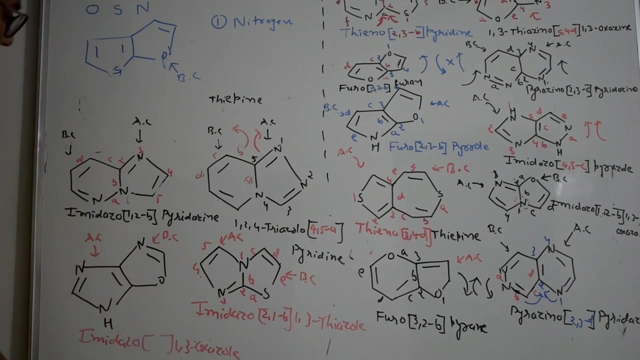 variety of heterotons. this is your attached component. so this is your base attached component. again one third position. so it's called imidazole right, and this is one third position. oxygen and nitrogen. so one, three, five. so oxygen will compost. oxizole right, 5-ohm bourdon is this. so let us give the your. 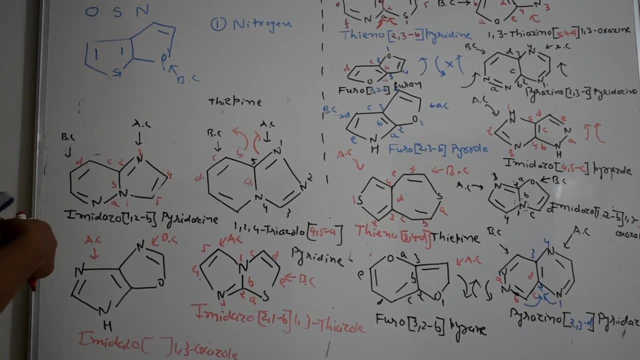 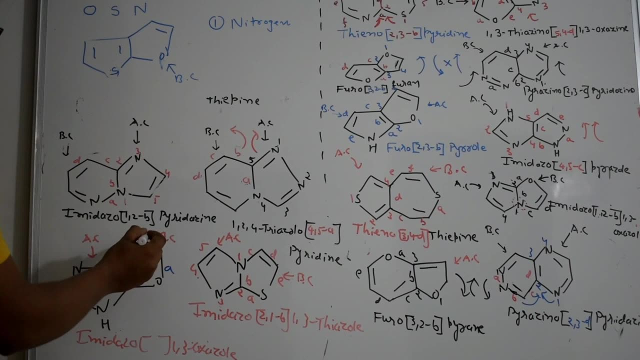 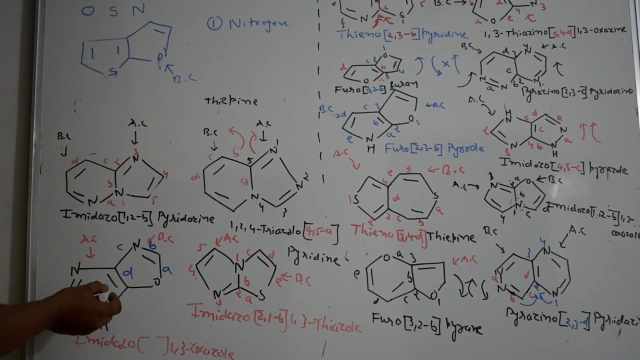 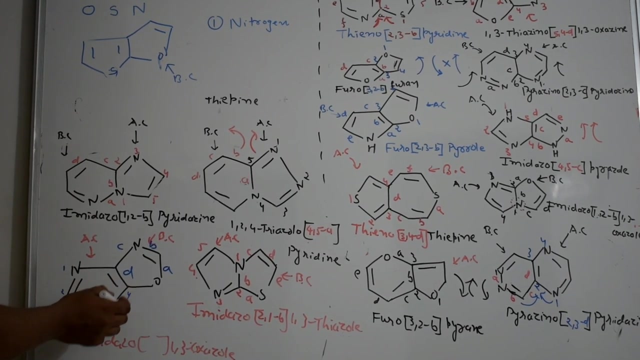 alphabets to the base component. so for the base component we can give the alphabets from this: a, b, c and d, and for your attached component i have to give numbering possible lowest numbering. if i will go like this: one, two, three, we'll get four. if i will go like this: one, two, three, we get four. but i will. 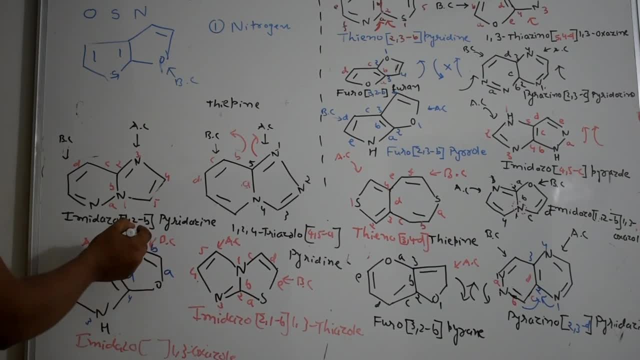 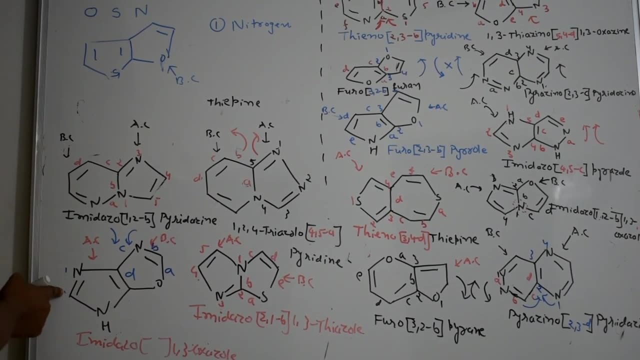 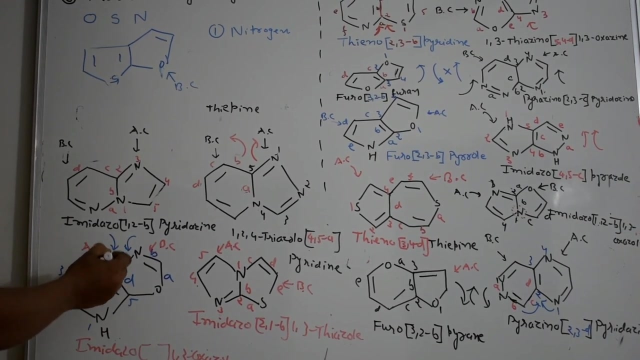 try to match the direction of your alphabet. your alphabet is going this direction, so i will try to give the numbering from this direction only, so the possible numbering so that go to this direction right: one, two, three, four, five. so i do not have to change anything because by the same way you are. 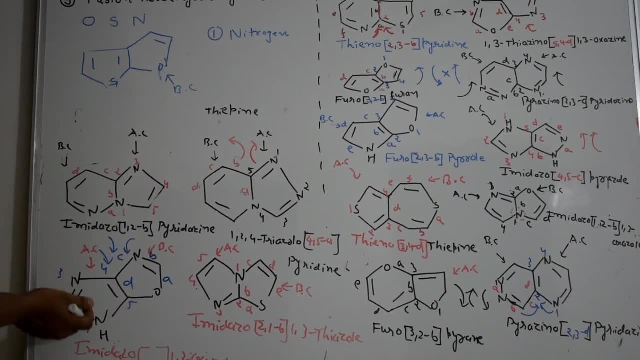 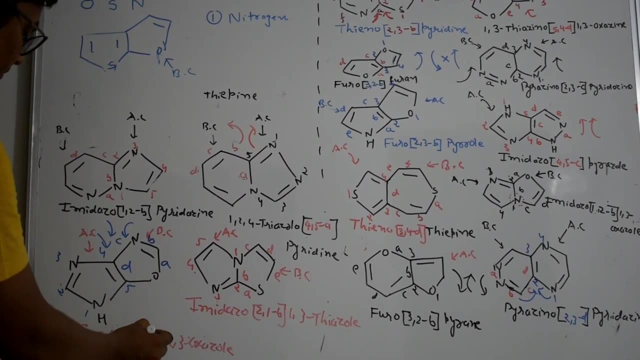 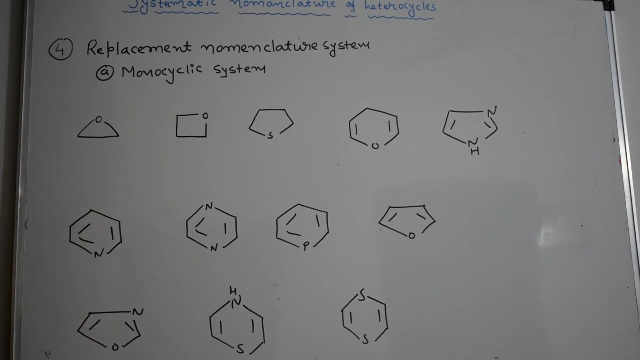 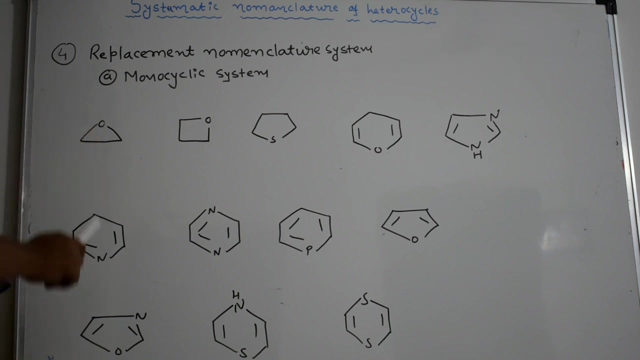 getting your, your heteroid is getting the lowest number. so i will say it's a four, five d, one, three oxyzole. so after your fusion nomenclature system, we are going to discuss the replacement nomenclature system and we will discuss the replacement. first we will discuss on a monocyclic system. so in a replacement monocyclic. 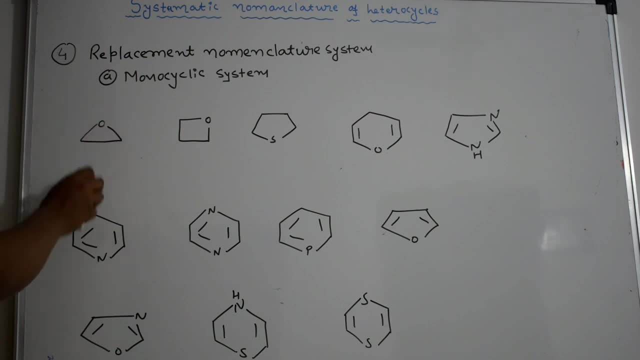 system, your all. the ring is considered as the carbocyclic. for the example, if i will say that, how many numbers of rings are there? so it's a one, two, three, right, so here there is one oxygen and two carbon, although it will be called as the your propane, right? so how it will be called? so it's a. 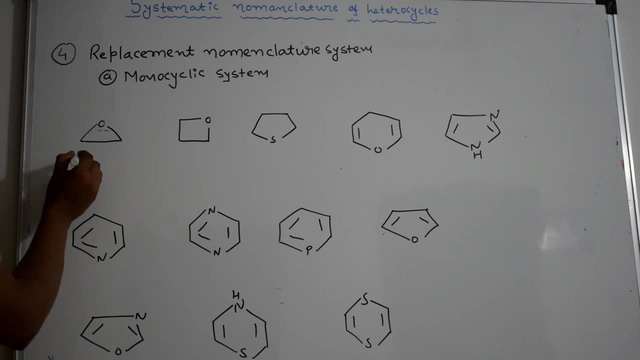 heteroitin. it's oxa cyclopropane, right. it will be called oxa cyclopropane, right for this. you can see how many numbers are there: one, two, three, four. so it will be called as cyclobutane and the oxygen is there. it will be called as a oxacyclobutane- oxacyclobutane. 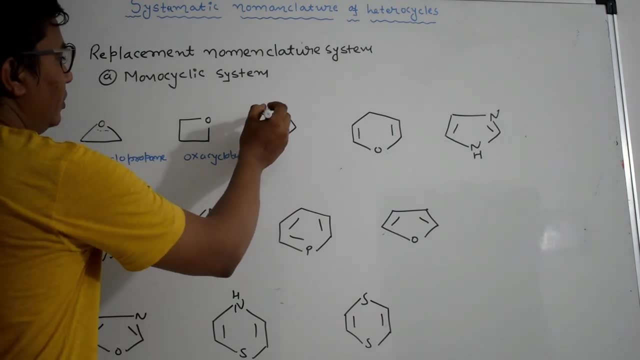 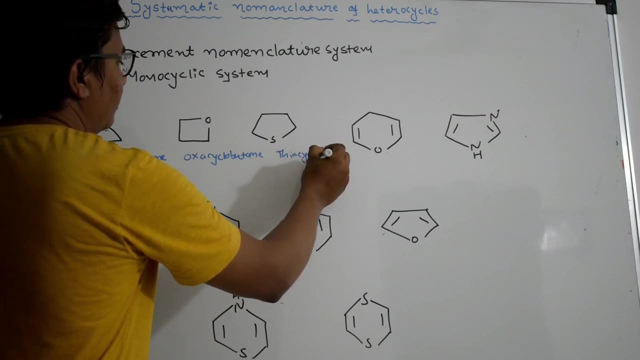 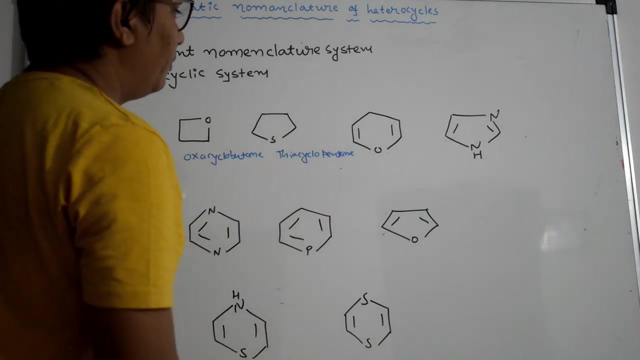 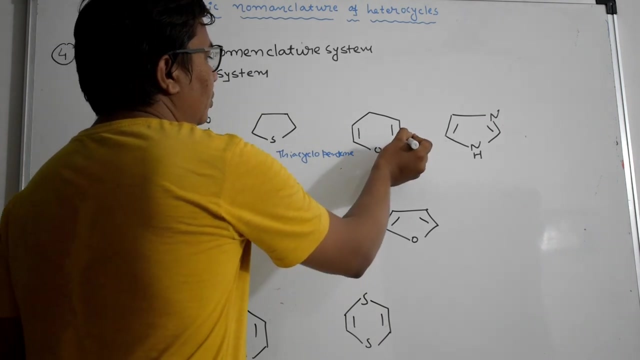 for this 1,2,3,4,5 number ring and there is a cell for that means thiacyclopentane, when there is unsaturation. so we also have to give the numbers to the double bonds. so I will start with the heteroatom. so 1,2,3,4,5 and C. 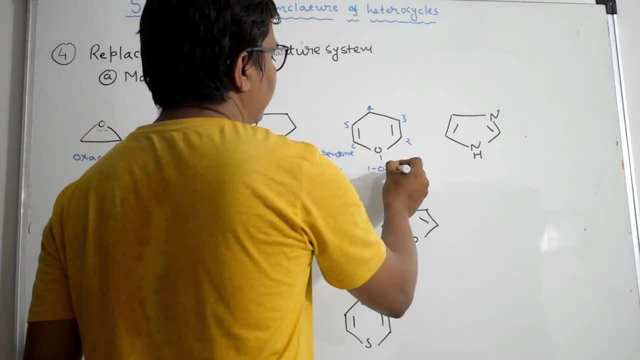 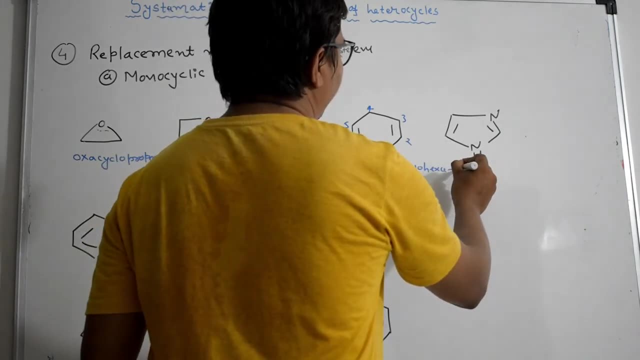 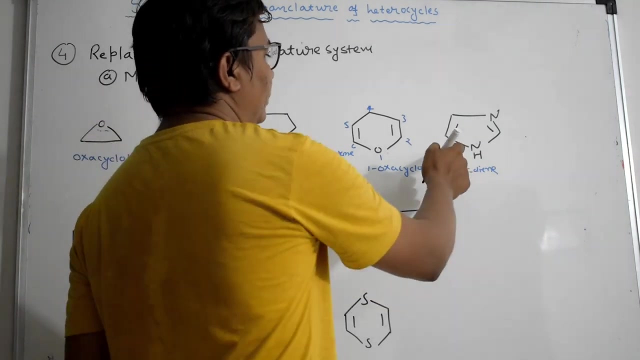 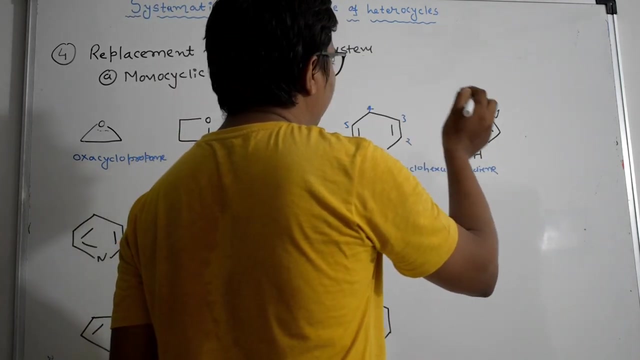 so it will be called 1-oxa-cyclohexa-2,5-diene. now for this ring. again, I will start with the nitrogen atom. so I will try to give the lowest number to the nitrogen atom. so the numbering will go like this: 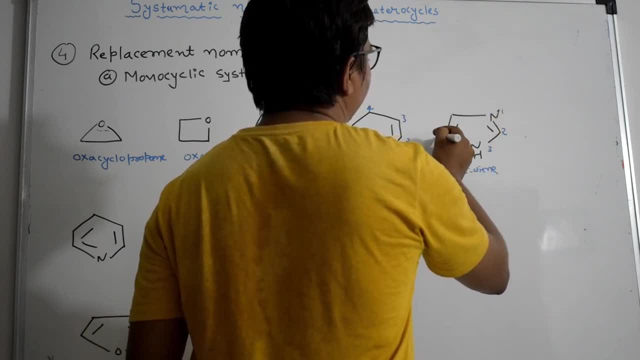 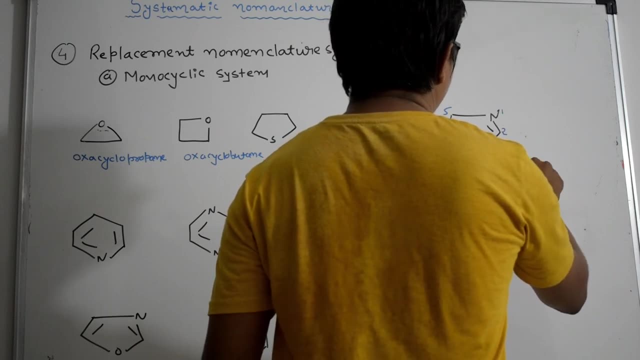 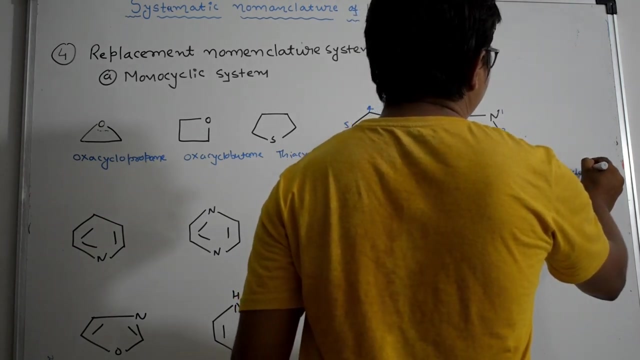 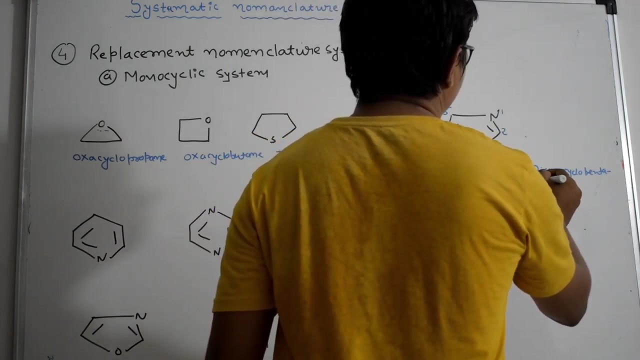 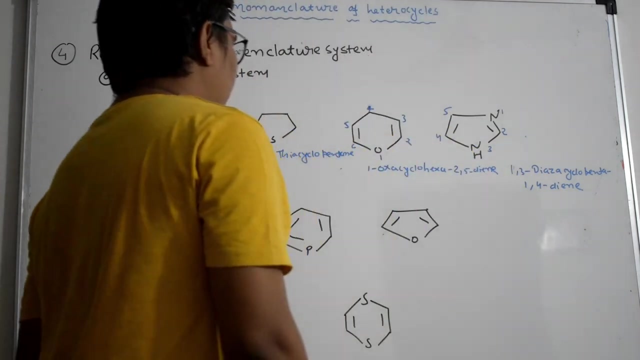 1,2,3,4,5. right, so it will be 1,3-di-esa-cyclopentane or cyclopenta. we can say 1,4-diene, 1,4-diene. now let us come for this example. this is simply called as eza- benzene. 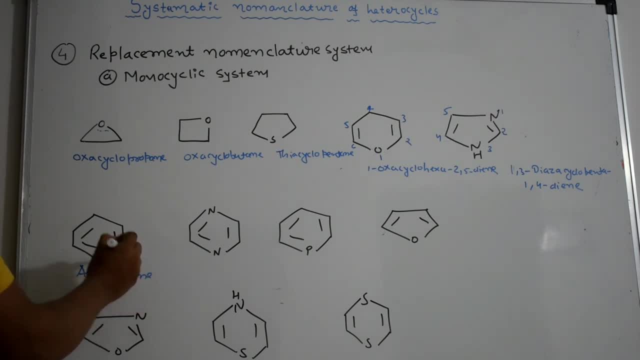 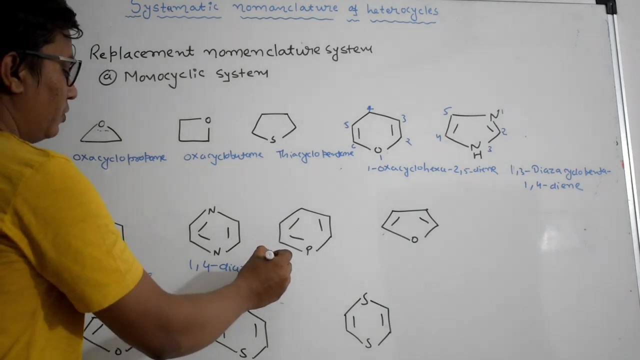 but this name is, I mean will not use, because, as we know that the driver name for this molecule is famous, it is pyridine. this will be called as 4-1,4-di-esa-benzene. and this name is also not used because for this molecule we know that the pyrazine is a private name. 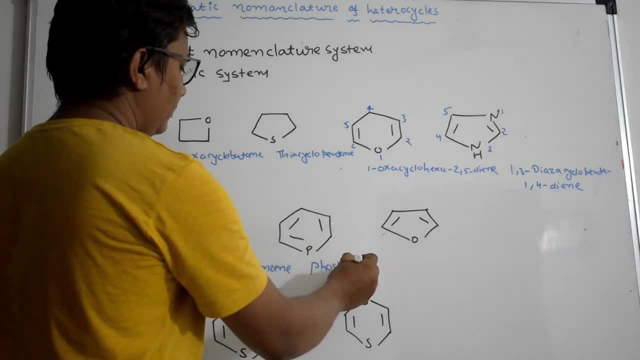 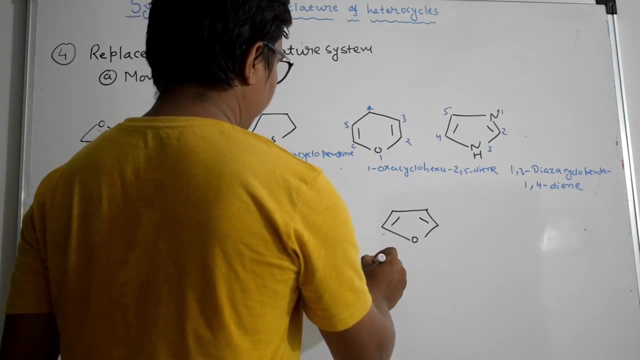 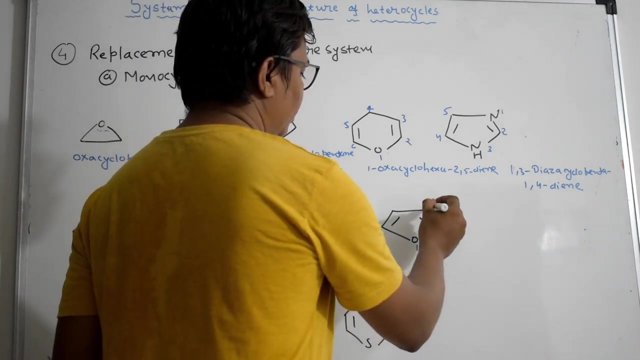 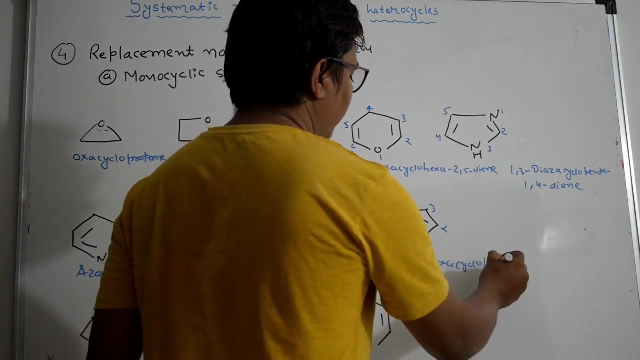 this will be called as 4-spa-zene, so 4-spa-benzene. now this one. you can see it is a 5 member ring, so I will say 1,2,3,4,5, so it will be 1-oxa-cyclopenta-2,4-diene. 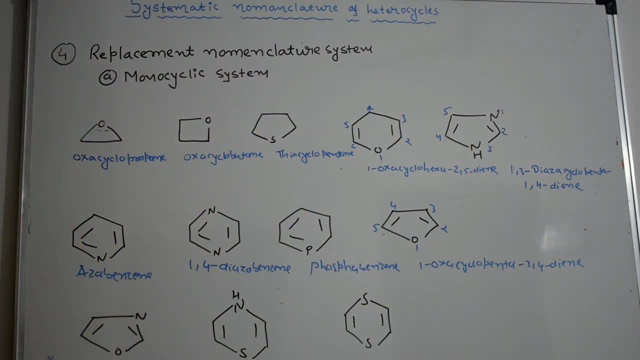 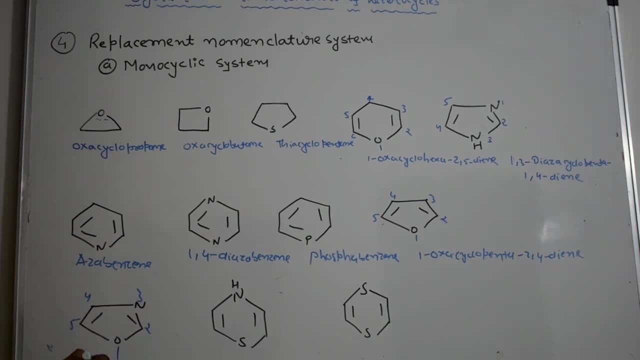 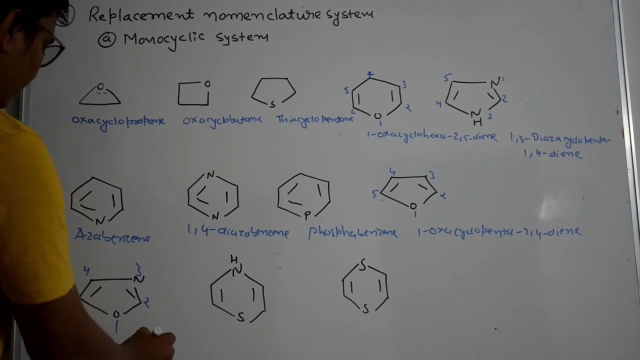 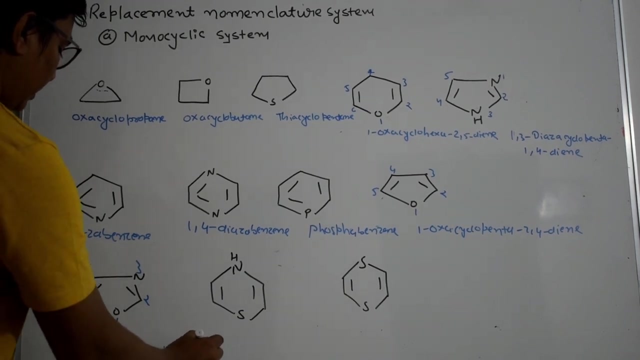 now let us come to this example. oxygen and nitrogen oxygen will come first, so 1,2,3,4,5, so here 1-oxa-3-esa. then your ring is a cyclopenta and double bone is on 2 and 4.